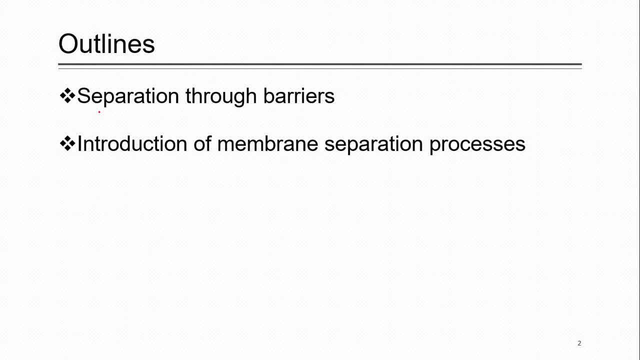 So in today's lecture we will start from very basic stuff, that was separation through barriers. so I will just go back to the lecture one and two when we started this Subject in the start of semester, and I will mean recall few things from there. And then we have to jump towards membrane separation processes. 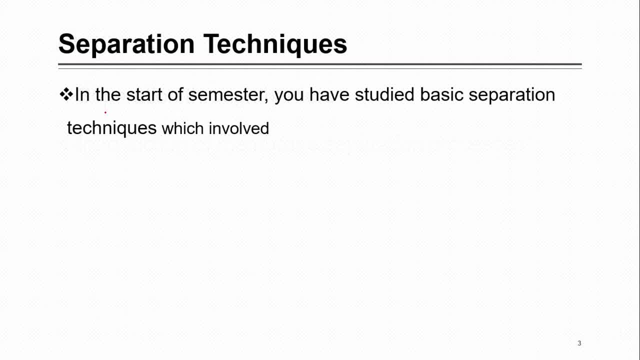 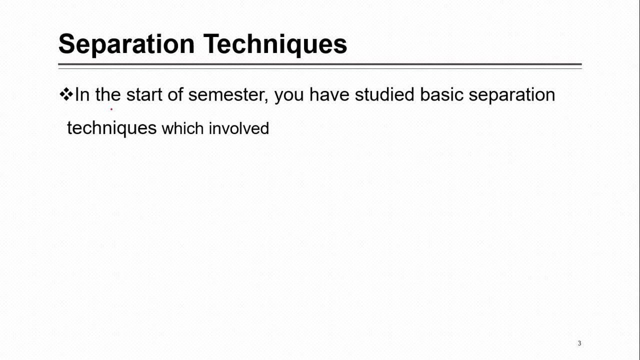 So let's start with this. So, as I said in the start of semester, you have mean studied Some basic separation techniques, that actually, when you go for separation, They can be classified or they can be categorized into four separate categories Or four separate techniques, and mean, when you talk, 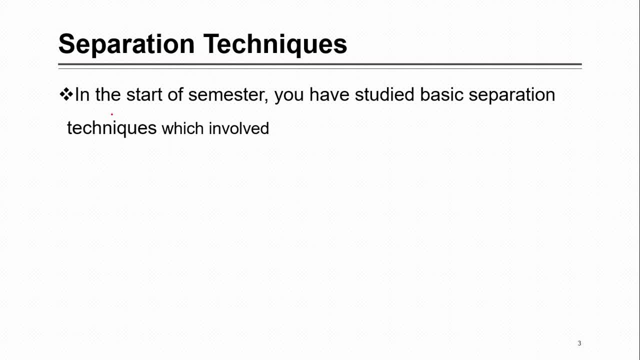 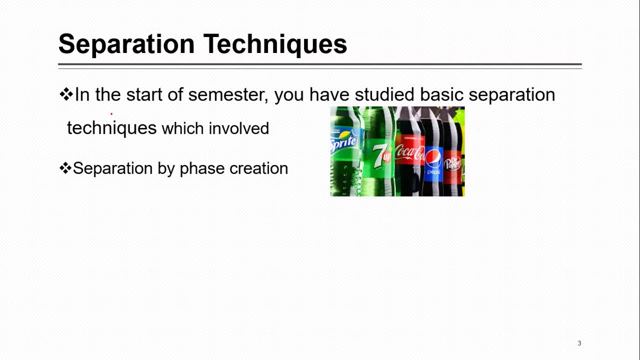 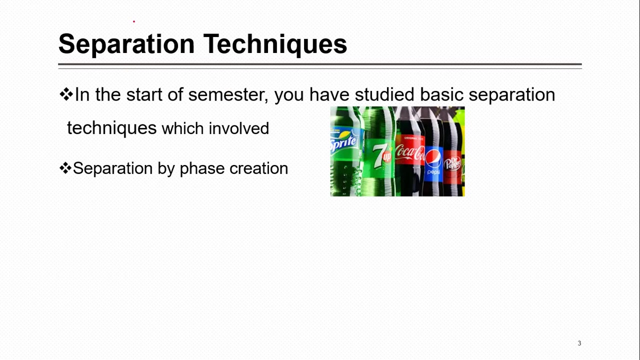 Generally about them. you can classify them in four categories and those categories Involved first one was separation by phase creation. and in separation by phase creation, This means that you have to create a new phase That Provides you separation of one component from the other. for example, here you can see these cold drinks in. 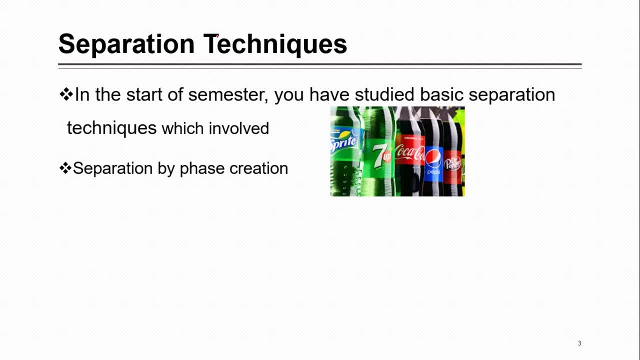 These- I mean this is very common example, Which you know, which we have also discussed in this- what happens when you open the main, this bottle? Actually, you release the pressure, you reduce the pressure and, due to reduction in this pressure, Gas, co2 is evolved from this liquid. co2 is actually filled with the pressure inside liquid and when you will open it, 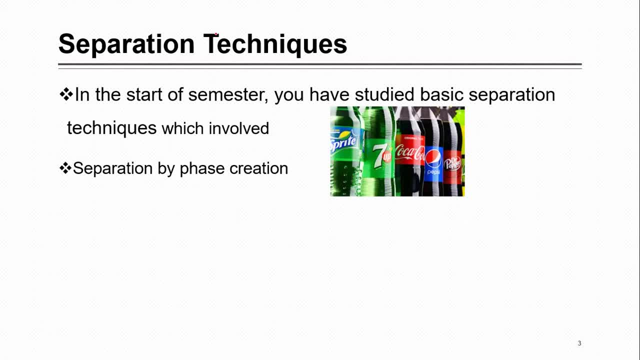 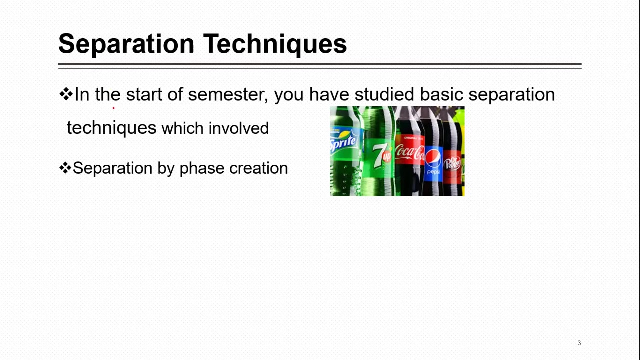 Due to this change in the condition, due to this change in pressure, This gas evolve and this formation of a new phase, that's that was dissolved here in the liquid But now that is released in the form of gas. This was phase creation and Related to this you have discussed or you know. the technique commonly used in the industry is distillation, in which you provide a 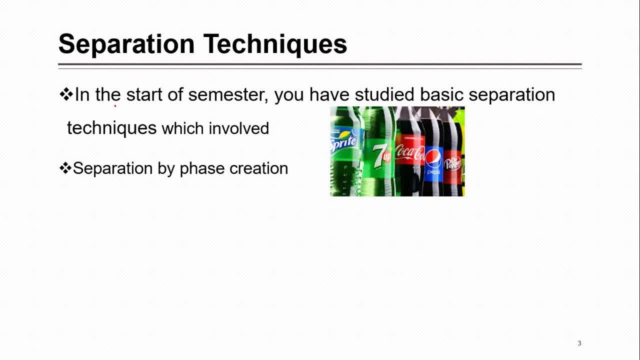 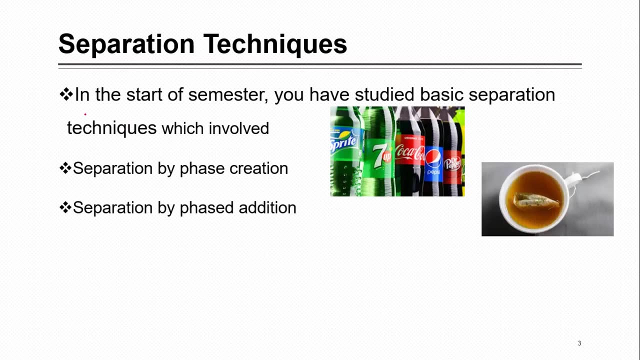 high temperature, and with the help of that you mean vaporize some part of your feet, while other is in the form of Liquid, and they get separated. So here, when you are vaporizing something, you are creating a new phase. So Next is separation by phase addition. 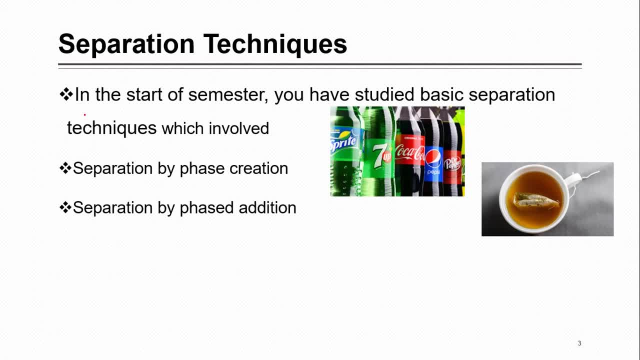 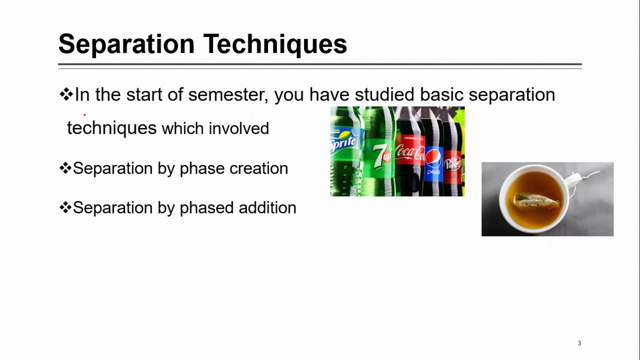 Separation by phase addition: here you will separate something by adding a new phase. for example, here very common example or simple example you can see- is like when we add hot water to the Mean, this tea beads or tea leaves. So what happens? some something is extracted from this solid beads towards water and 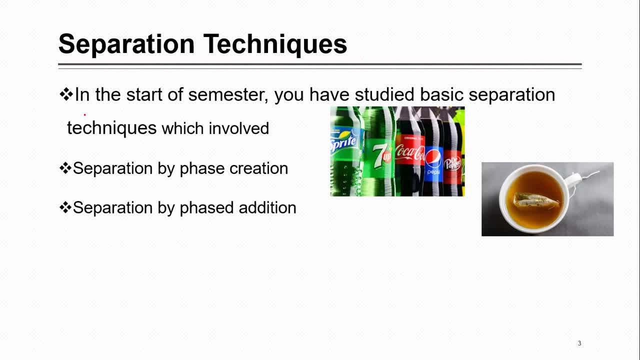 in. Similarly, there are some other techniques on industrial scale which you have discussed, and they involved actually Absorption in absorption- you remember that we discussed the topic in detail and you always introduce some solvent for removal of some components from the feed. and then, after this, we discussed 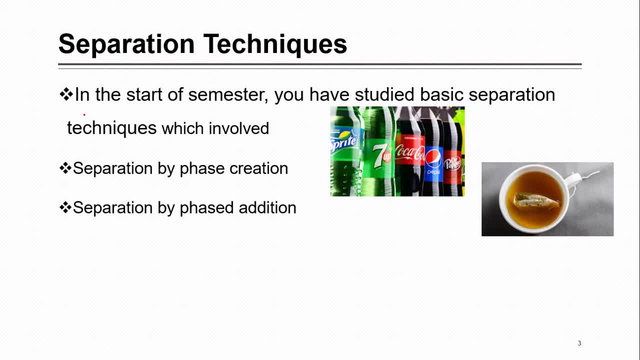 Man in last few weeks: Liquidity, good extraction. So what we were doing there, We were introducing some new liquid and that was like phase-new, phase addition and with the help of that, we Separating some components of our feed That was solute, which you were mean. 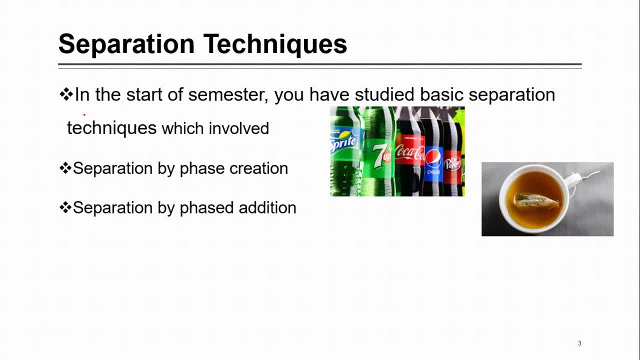 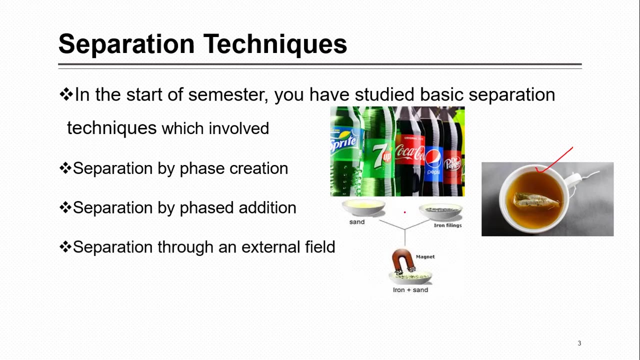 Extracting with the help of externally introduce solvent as well, one technique Which still we have to discuss at the end of this semester as well, and that is leaching extraction. And this example of T is actually the solid liquid extraction, because we are extracting something from the solid that is beat with the help of some liquid. 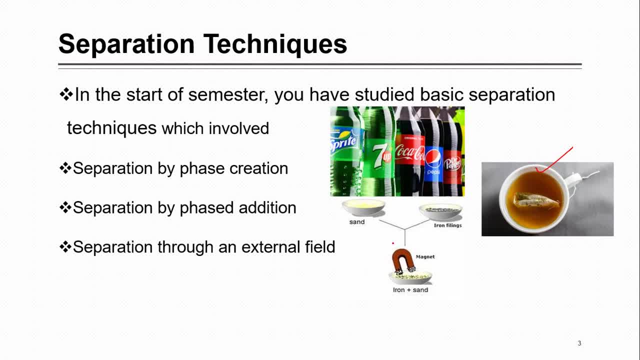 And then there is separation through external field, in which you apply some external field and you get separated some mixture. So in this example, which you commonly know from the FSC class, this being used here and some technique which on industrial scale is used, called electrophoresis, I think we discussed in the start of semester, which is usually 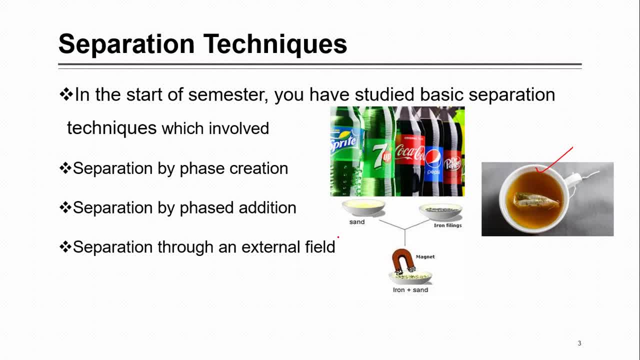 used in some how nuclear industry I think, and they are used. they are externally introducing some fields. So here external introduced field is magnetic field and with the help of this you can just separate iron fillings from sand Like new phase. you did not created any phase, but what you did, you applied any external 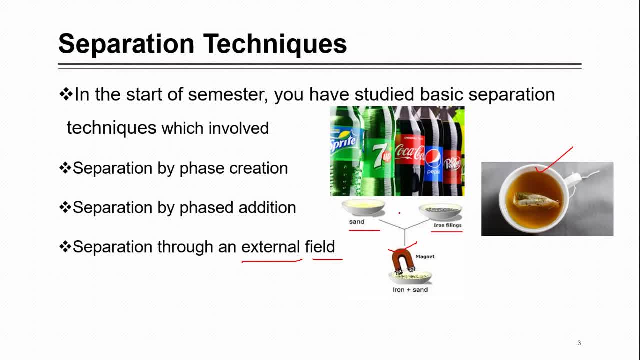 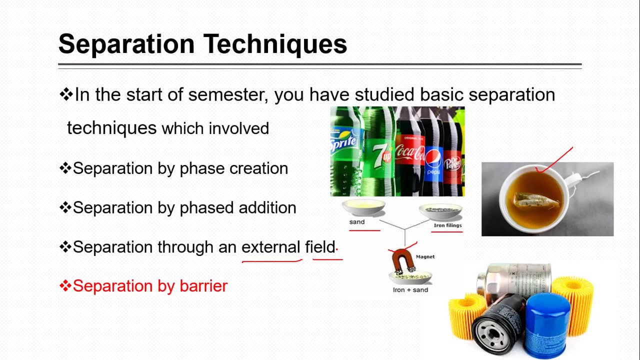 field, external force- and with the help of that you have separated a mixture. And then there was last type four, technique or fourth category, and that was called separation by barrier or you can call it separation through barrier. In that we discussed various example I have in the news next slide: 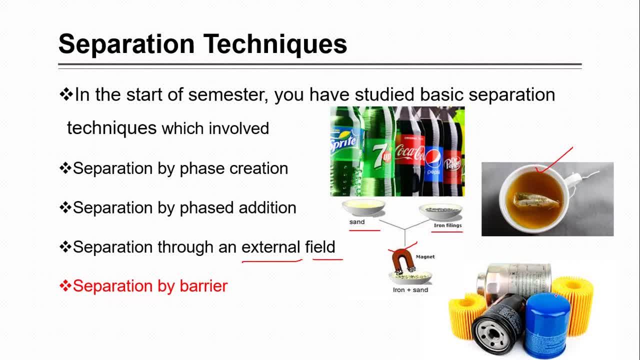 So here you can see these are called filters. some are air filter, while other are oil filter. we discussed this example there. So in this, what happens actually? you are separating some components from the others with the help of some barrier. For example, if you talk about 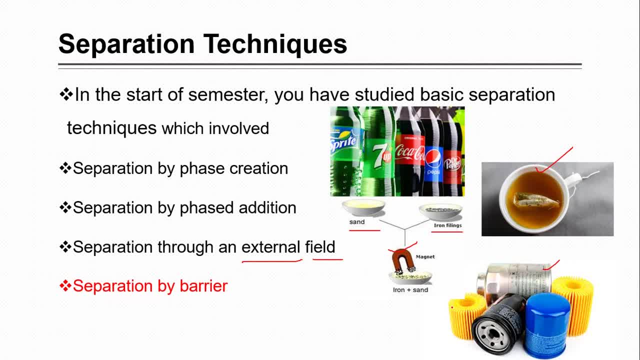 air filter. what happens? air which is going to enter to your system, to the engine. So that is mean we just purify that air. So dust particle, other means some, something like if there are some particles which can go to engine and can damage that, they are removed with the help of this filter. So 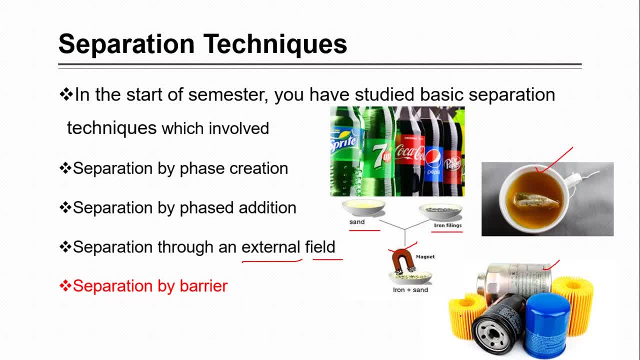 when air will pass through. air will go through, but those solid particle are trapped inside this barrier As well. if you look at these oil filters- So oil filters- we remove some solid particle present in the oil So it did not damage the parts of engine through. 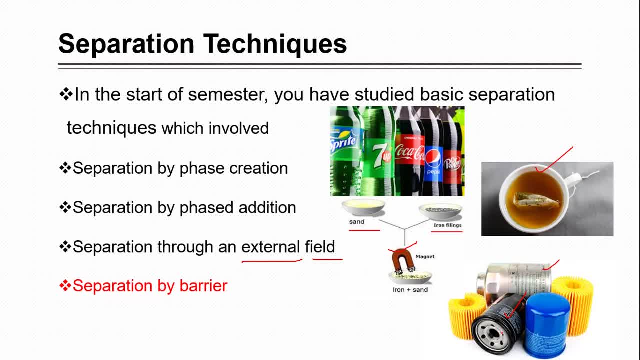 which this oil is being circulated. So when you will pass that oil through this, these oil filter contains such structure inside that that will allow only oil to pass through, while if there are some solid of some specific size, they will be trapped inside this filter. 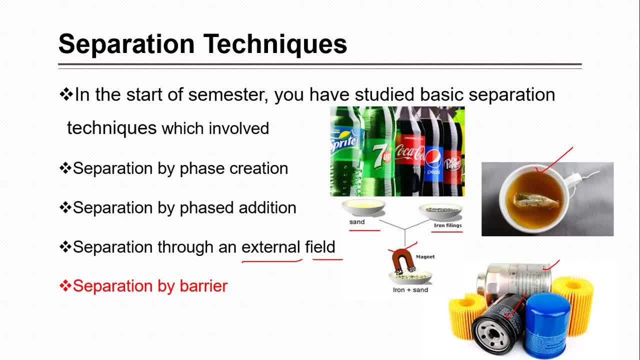 So in clean oil, will be moving towards your moving parts. So we have to actually take this separation by barrier and discuss in detail. So, through separation through barrier- yes, before that I jump toward next slide. So if I talk about the industrial example, about this, So that is membrane application and 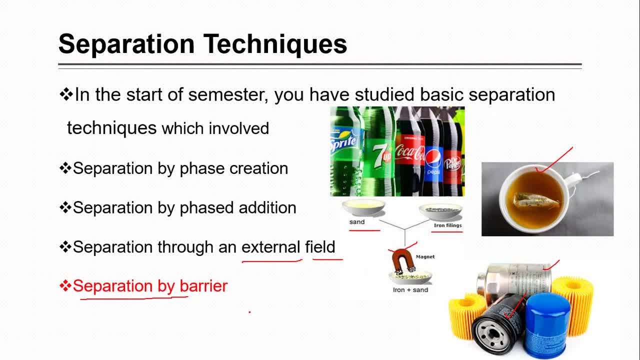 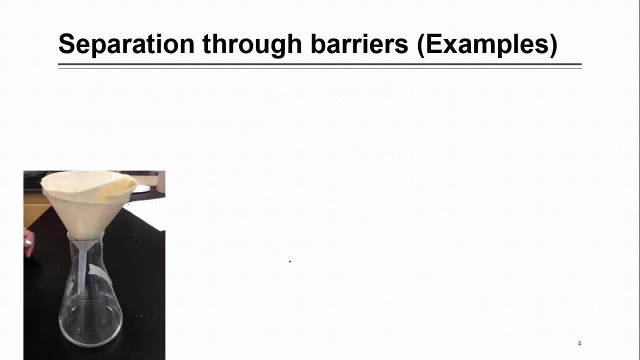 there are various type of membrane application which come under the category of separation by barrier. So there were few common example which were discussed in the start. So you can see here this example which you commonly use in lab mean when you are separating. So 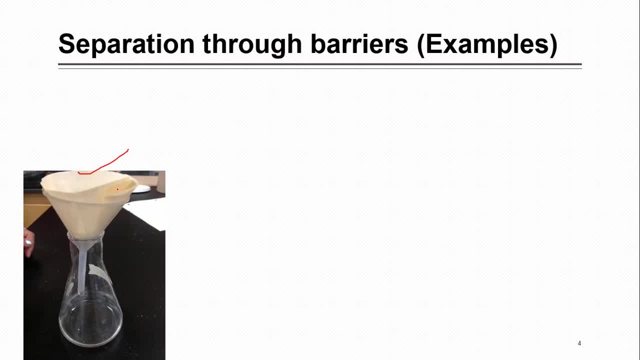 some solid. you go for crystallization and for various analysis in chemistry when you go through this. So here what we do, we will just pass in the liquid and solid, some, I can say, mixture, through this. So when it will pass through this, you know that solids are retained and the surface and liquid will pass through. 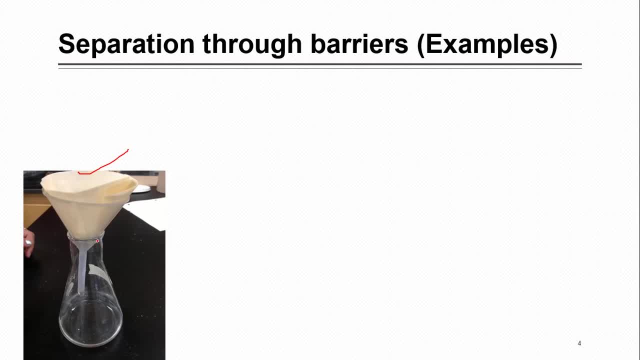 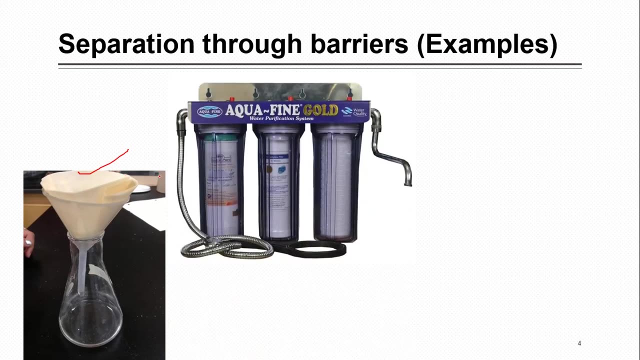 So this is just separation through barrier. we did not introduce any new mean phase, we did not create, but we did. we did not apply any external force here, at least in this case. So what you did? you just provided one barrier and separation takes place. Then these water filters you. 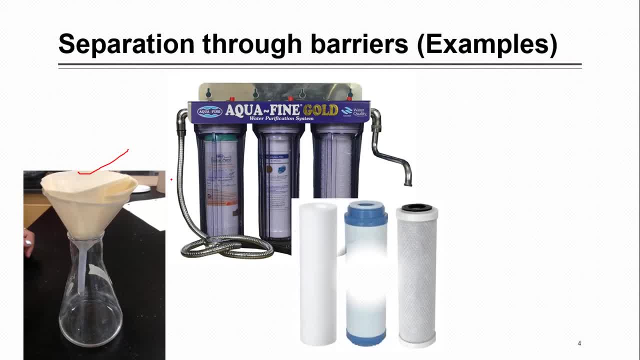 commonly know that they are used and here they actually contain some. the filters of various sizes are various material actually, and they capture the solids of various sizes through the water So that we can we can get, at the end, clean water. So this is again. 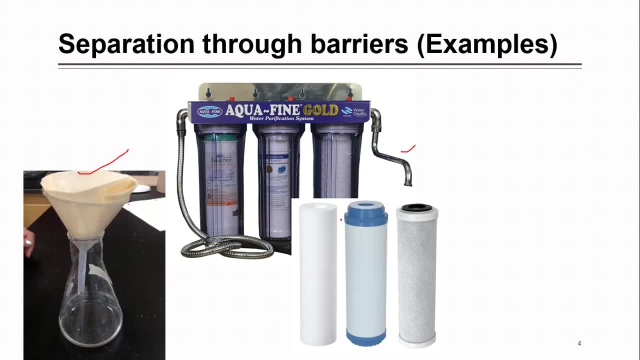 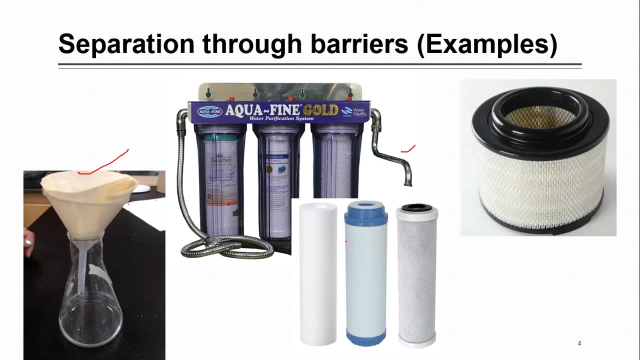 the separation through barrier, in which you are applying one barrier which is a filter and based on particle size it is making separation And then this is, I think, air filter. So in this, when you pass air through this air will just get separated because air will pass through but the solid particle are untrained on the 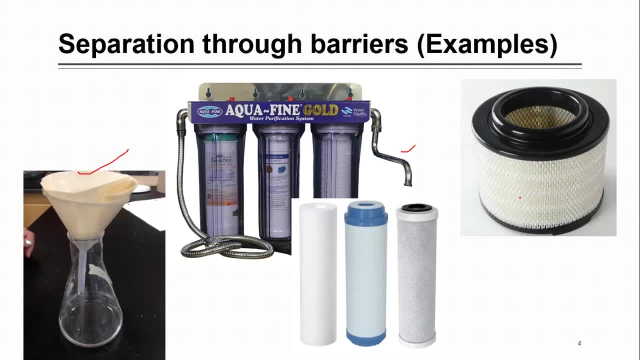 surface of this. either I mean inside or outside. So those I mean. it will depend on the direction of the flow, from where you are flowing this air to. in which direction, suppose I am just air is entering from inside and leaving or pushed outside, So all those particles will. 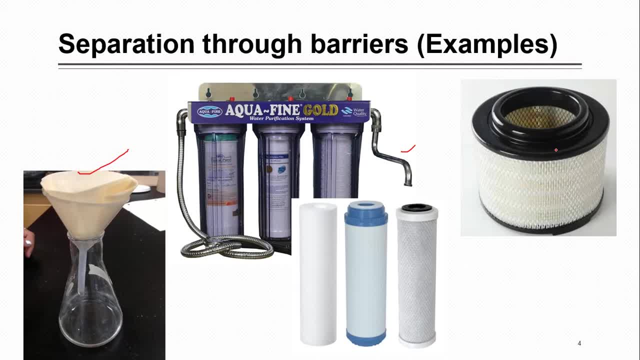 be entrained inside, and if you are pushing air from outside towards inside, So here then solid particle will be, I mean, entrained on its surface. So all these are example of separation through barrier, but they are being used on small scale. So if we have to talk about on large scale, industrial scale, So then there is 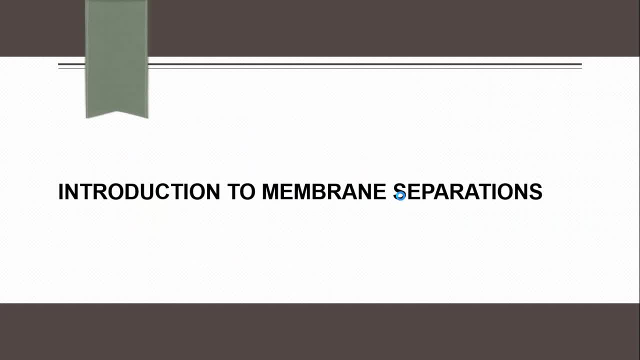 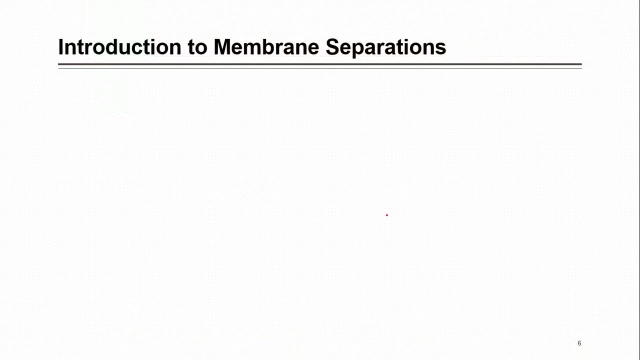 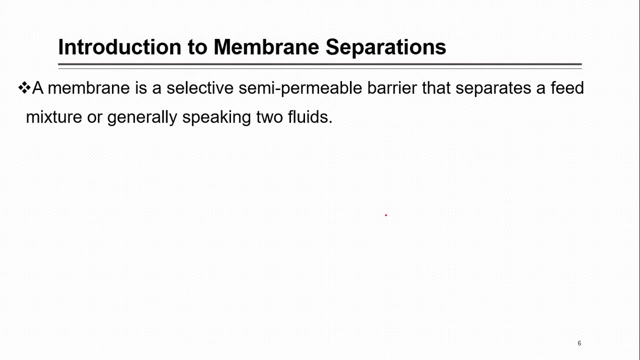 example of actually membranes, that is, I mean separation through a barrier. membrane can be considered as a barrier which will allow the separation of various components of the feed. So let us look at this. I mean membrane separation, Like when we say membrane separation, as I said in last slide, that this is separation. 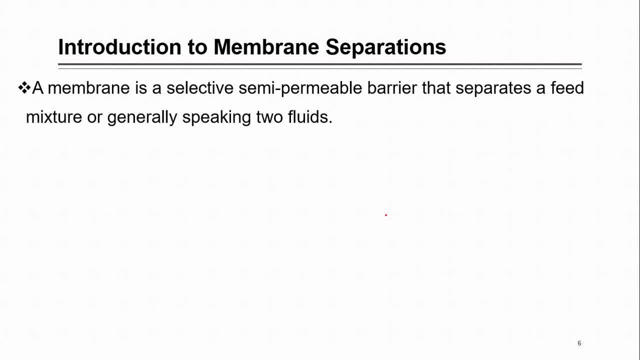 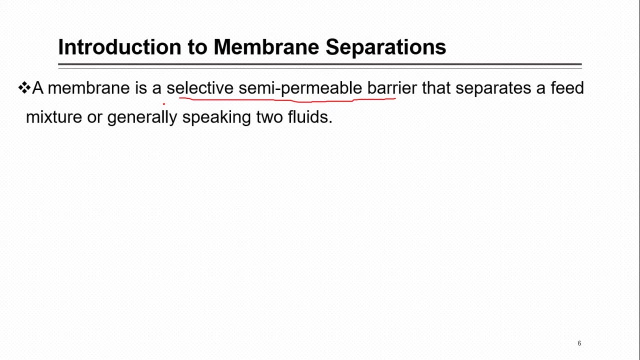 through some barrier. So that barrier is working in such a way that it is selective towards some components, or it is like selective semi-permeable barrier, So membrane actually can be defined as selective, semi-permeable barrier that separates a feed mixture. I mean. 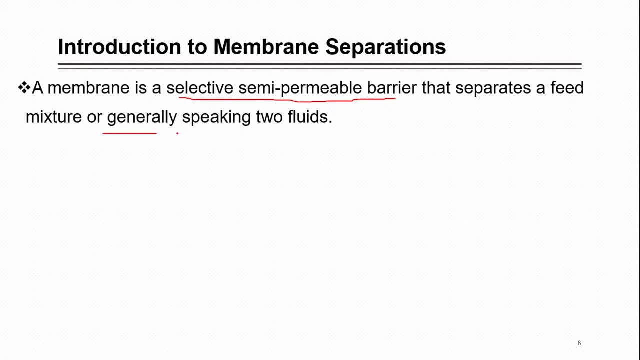 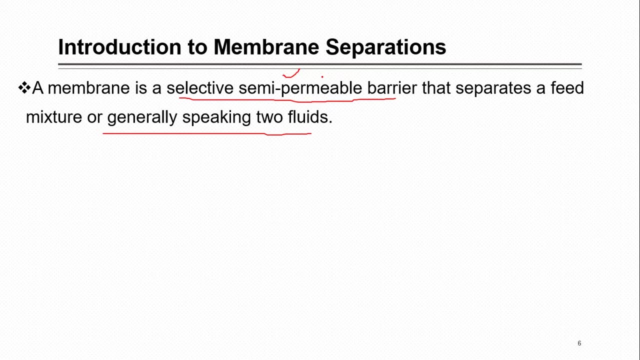 into its component. or you can say, generally speaking, if I just say there are only two fluids inside my feed, So membrane is a semi-permeable barrier that will separate two fluids into two streams. So this semi-permeable- something which is like selective for some components- 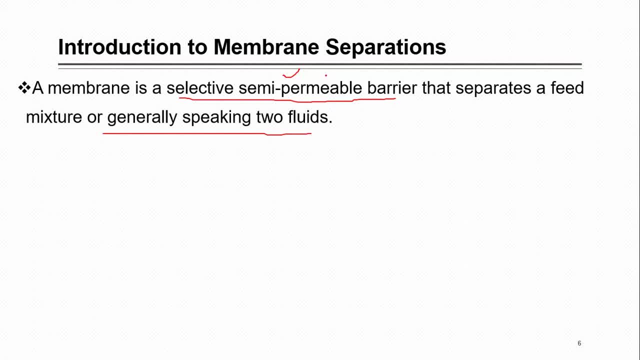 which allow some components to pass through, while other will be retained on its surface. So this you can compare now with those which we have just discussed, that they were also allowing some of the component to pass through while others were retained, For example, you. 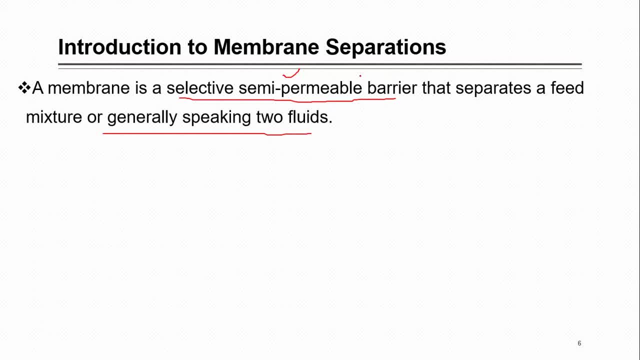 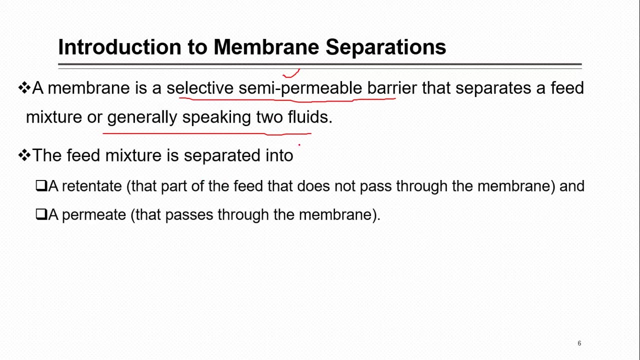 have water filter that allows only water to pass through, while other solids or some impurities present in that water are just, I mean, retained on the surface of filters. So here the same methodology will be applied. So overall, when we say that, I mean feed in the gas is separated into two parts, like actually. 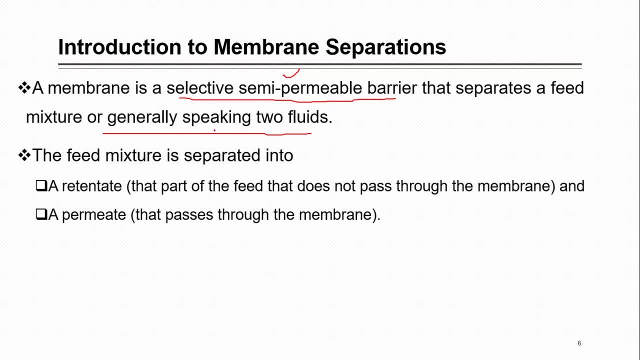 one part will pass through the membrane while other part will be retained on the surface of membrane. So they are given some specific names in the field of membrane separation. So they are called actually retentate and permeate. Retentate is that part of the feed that does. 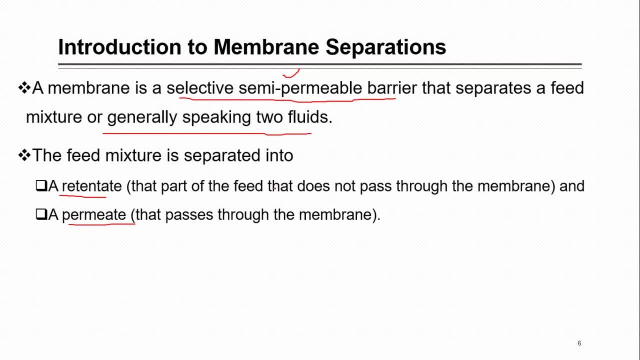 not pass through the membrane is named as retentate. something which is left over, which is not allowed to pass through, is called retentate, And while there is something called permeate. So permeate is that passes through the membrane, if you look at the meaning of this word permeate. 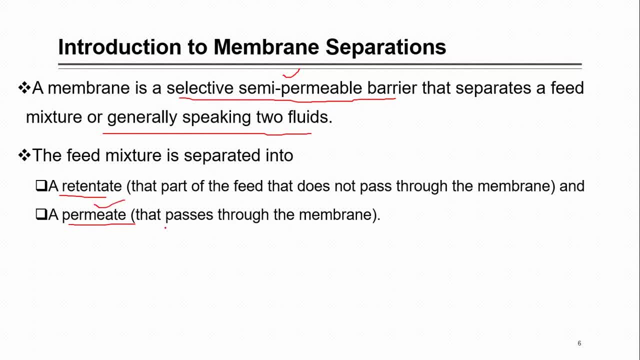 pass through, that will. something will pass through the membrane that will be called as permeate. So when our feed will be entering to this system, for example, here you can see that we have a feed and that is a mixture of, like here, two components. it is not necessary sometimes. 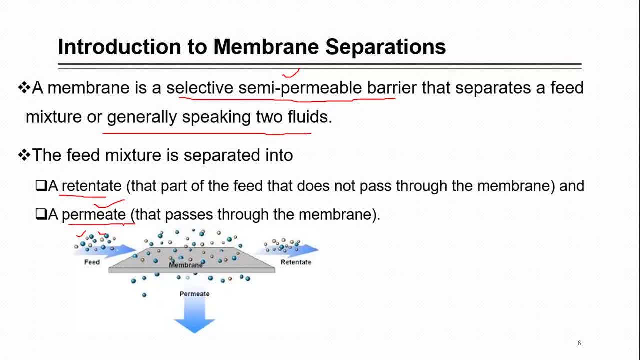 we can have more than two components, So our membrane will be selective for some of those. and we have to select such membrane that it mean it gives us separation. For example here mean two fluids are present and it is separated. 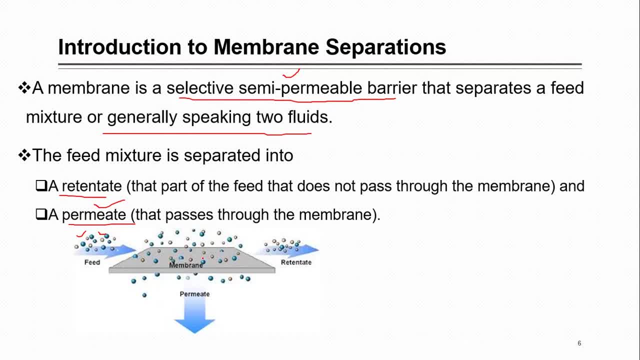 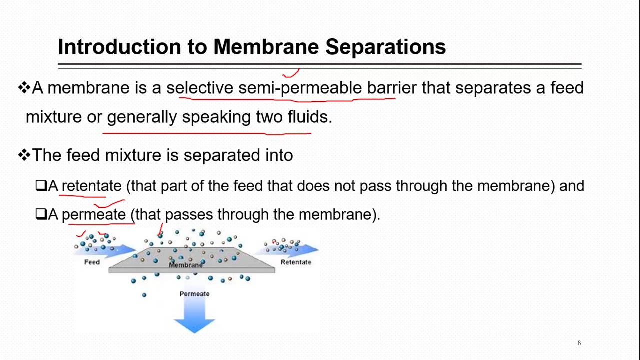 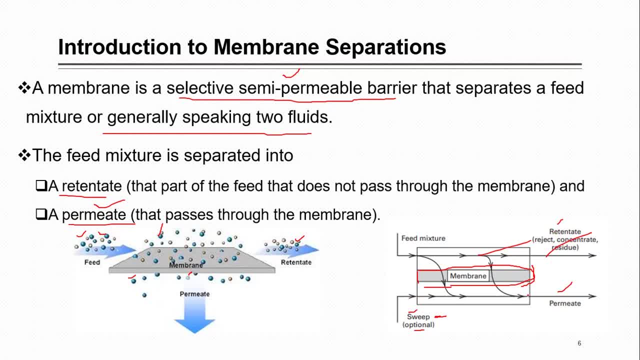 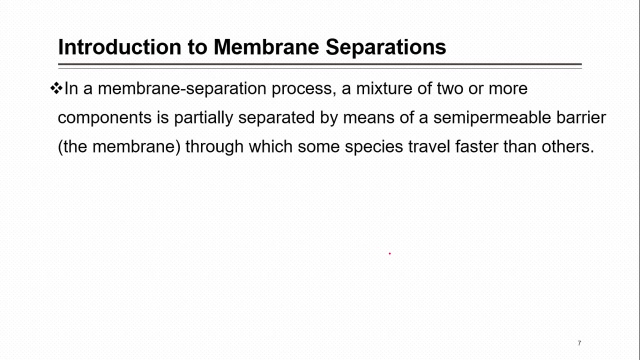 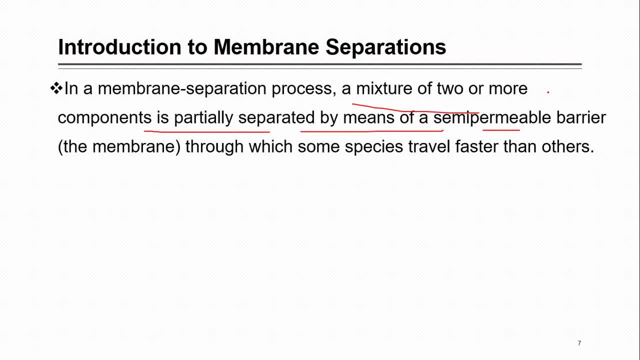 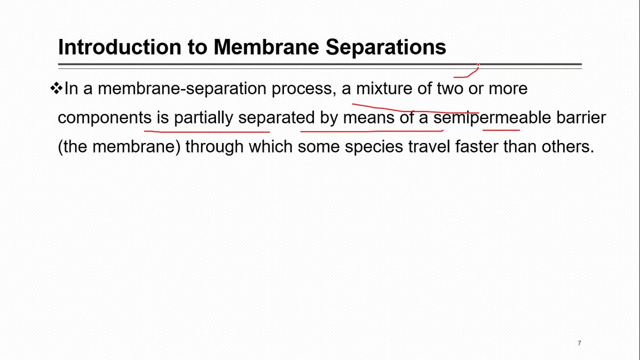 And later we discussed this topic. Sosometimes you have more than one membranes in series, so to remove various component are you can have more than one means set up in series So you can remove more than one component from your system. 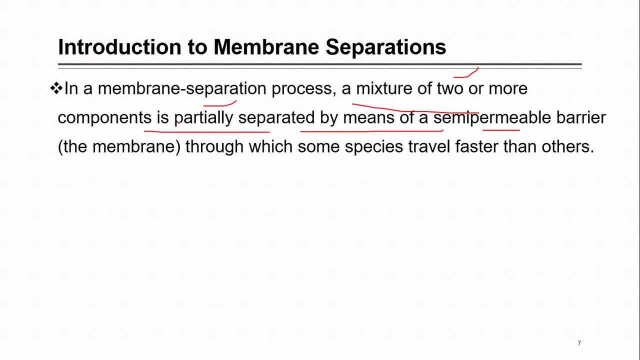 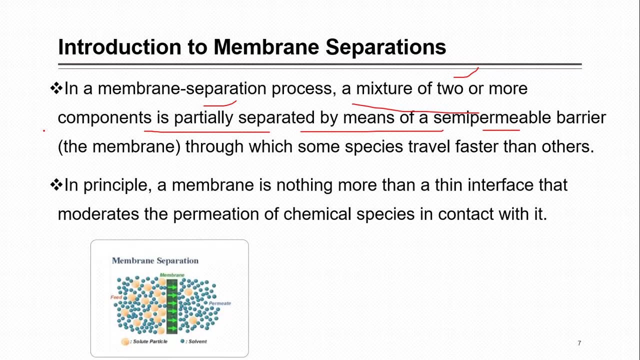 As well. something, one thing mentioned here is partially separated, Sothis islike not 100 percent separation. definitely few of those are still left with each other like here. you can see somehow in this figure overall- just look at this- that this was a mixture. this was. 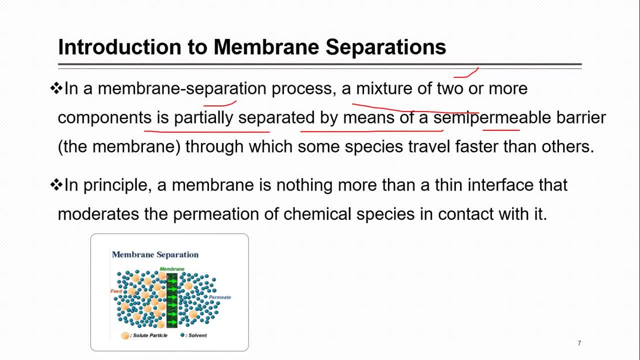 the feed and if this feed is passing through this, so here somehow size based separation is taking place and small size particle are passing through this, but as well you can see that some large size particle are also passed through this membrane. so this is like partially separated, not hundred percent separated. 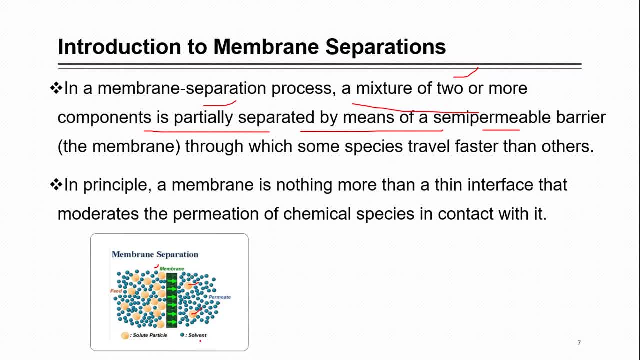 so overall your solvent and some solute particle are there. so solvent will pass through more or less almost all, but other solute will also pass through. but at the same time this is permeate if you will look at the retentate, pure retentate. 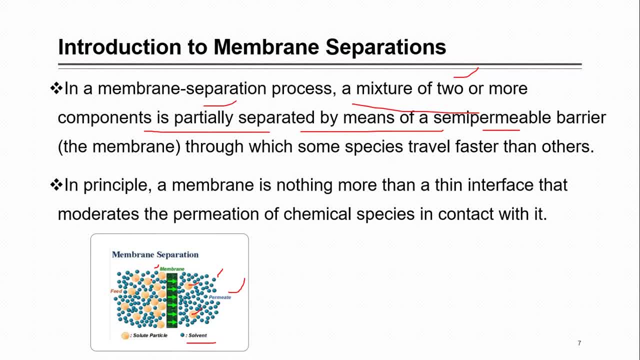 will also contain some of the solute mean. hundred percent solute is not separated, so that's called partial separation. then if you look at these membrane mean they are nothing. they are more, just nothing, more than a thin interface. thin mean, like you can see, that has very 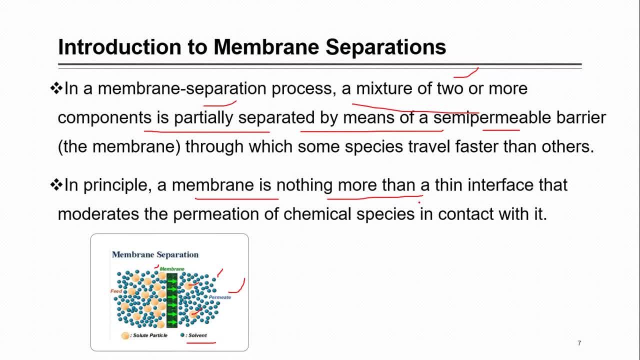 small diameter actually and very some small like sheet. you can consider it something like page, as I told you earlier, somehow somewhere that they can be considered as a one page like, as you have seen, filter paper. actually they are just that can be treated as a membrane, but here actually membrane assembly. 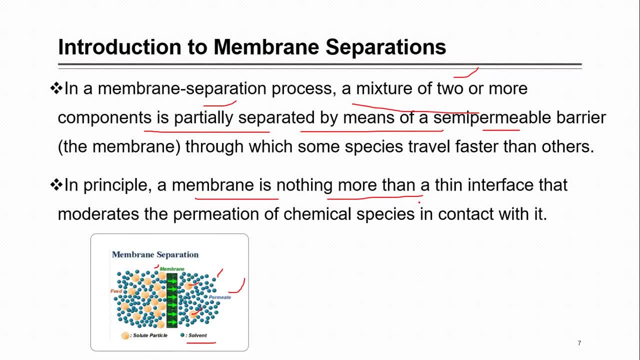 namely, is not that simple. that is not only one sheet or one page. they also involve some others. I mean structures which are used for helping or may be supporting your, this thin sheet. So actually, what happens on the surface of this thin interface, interface is actually. 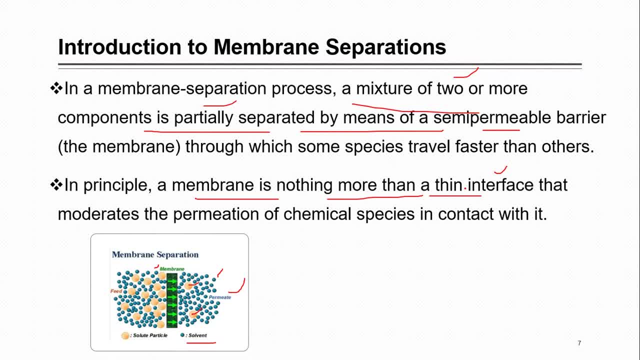 that point where something separation is taking place or some of two components are just, I mean getting closer to each other or coming in contact with each other and, like you have seen already, some we call interface that there is a interface. interface is actually in liquid, liquid extraction. when we were talking about this, 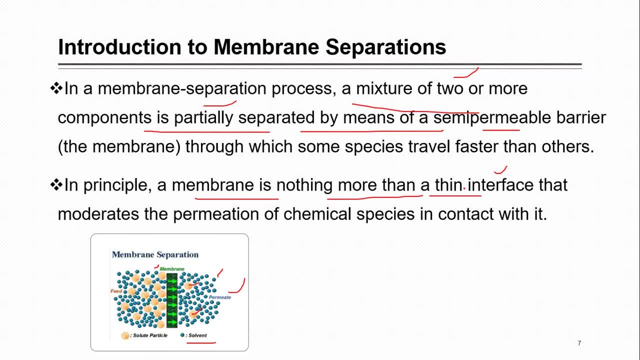 So that is, I mean some two of those components are coming in contact with each other, as we were bringing our feed And solvent in contact with each other. so some interface. there will be some boundary actually where their contact is taking place. So here this is thin interface through which actually separation is taking place that moderates. 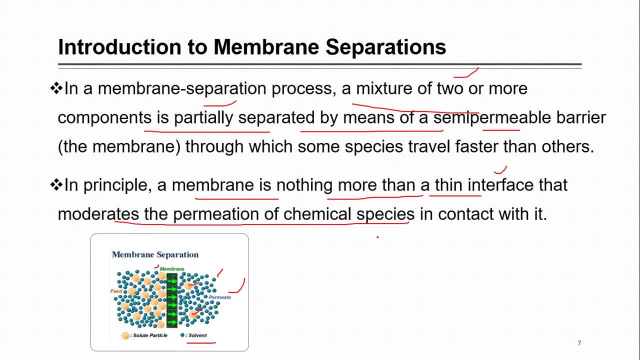 the permeation of chemical species in contact with it. So permeation, this is from permeate, so that allows or that moderates the passage of some chemical species which are coming in contact with this Suppose. here we have some. So somehow the similar example, some feed is moving through this. you will look at this. 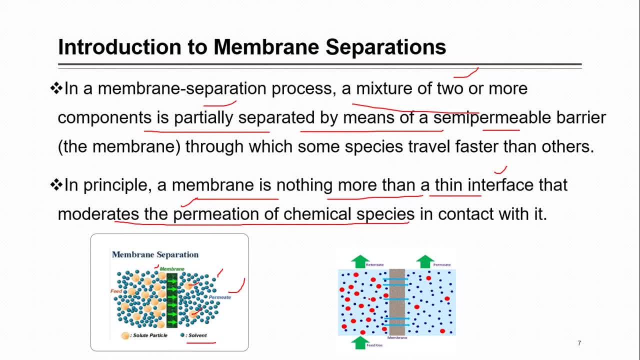 membrane later, like there are various type of setup or assemblies through which we can pass our feed and get it separated, So overall some of those component, while this feed is passing through this in this direction, So some of those component will travel or will pass through, will permeate through this. 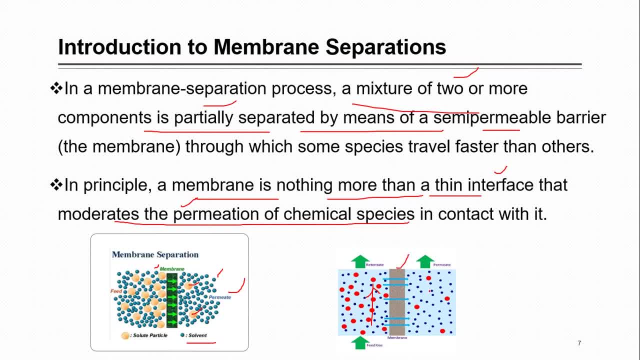 membrane. this is membrane barrier, So they will go on the opposite side and that is called then permeate. So this is something which has passed through the membrane is straight named as permeate, and while other which are not passed through this and they are still left as such when 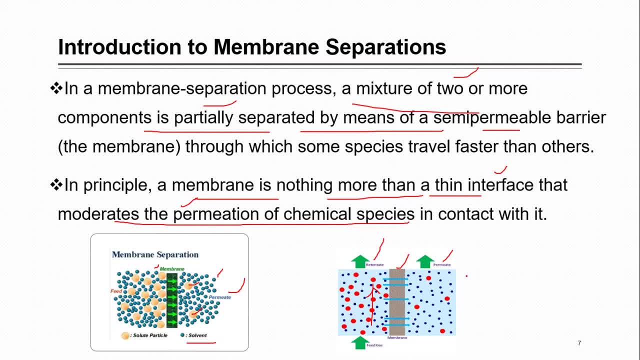 it is leaving this system. So that is called retintate and here you can see that this membrane again has allowed some of the red colour particle to pass through this membrane. Overall this is highly selective, or more selective towards this blue colour, but some of these 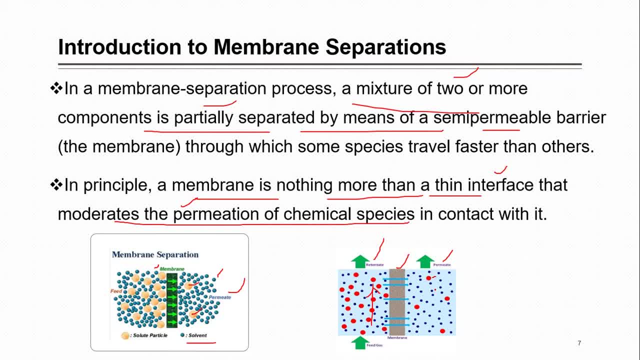 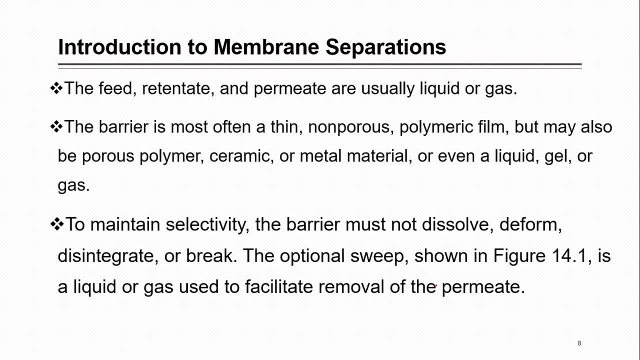 red are also. I mean pass through this, Thank you, Thank you, Thank you. So, overall, when you look at these membranes, mean these membrane as we are giving some feed and we are getting some permeate and retintate, So that can be like usually they are usually liquid or gas- mean, when we apply this membrane? 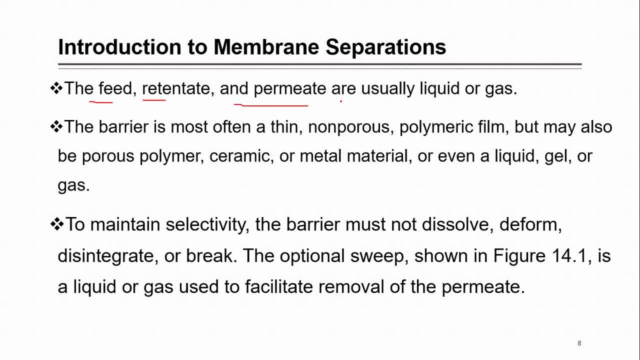 for separation. So they are commonly being used for liquid or gas separation. actually, I mean, here they are not commonly used for somehow you can say solid separation. So they are used for liquid or gases, but here what will happen in liquid? actually you, 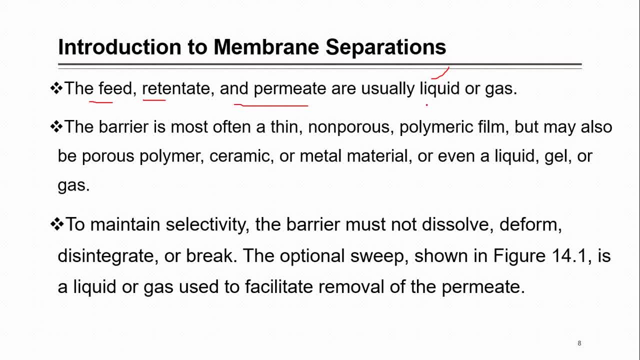 can have various chemical like, for example, there are salts. So you know salts are solid but when they are dissolved in the liquid, So that is, they are the part of that liquid stream. actually, So as well some other chemicals suppose, as we were talking about the water. 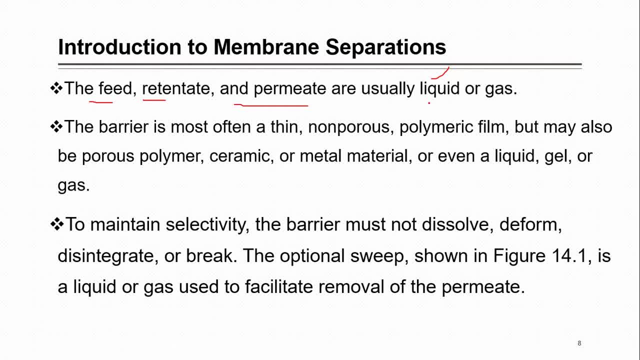 chemical like benzene, toluene- some of those are present in this, so they are part of this liquid stream. So when you talk about the gases in gases, like we can have a mixture of natural gas, when I think we talked about this in the start as well- that when you get this natural gas, 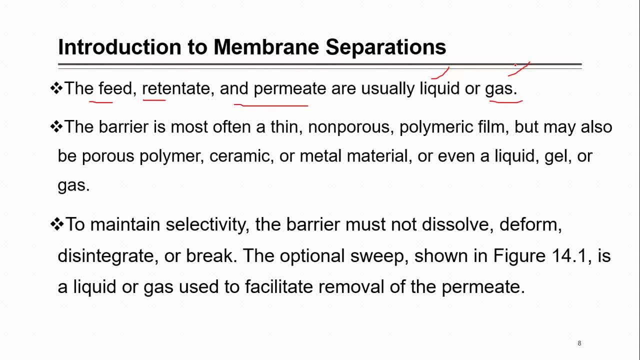 from the ground. so it is not only CH4, it is a mixture of various other species. like there will be CH4, there will be as well water inside this. some other gases like CO2 and H2S are present, So I mean that water that can be removed from this in the form of condensate, you can. 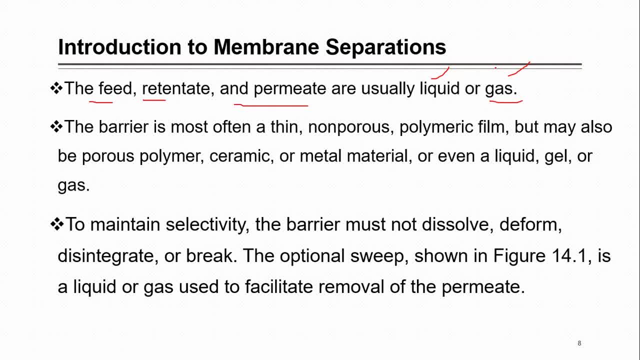 just condense and when you will reduce the temperature, definitely water will condense out. that will be separated. but these gases now, as I said, this is CH4, it contains some of other hydrocarbon like it also contain, you know, like after methane, ethane and butane. 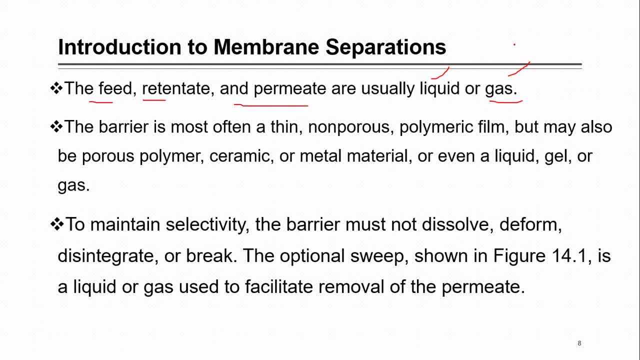 somehow propane are there, H2S and CO2 are the major impurities which need to be removed from this. So this is the gas mixture when we will pass through the membrane. so that membrane should be selective, such that I mean it separates these. that can be separated in two ways, like 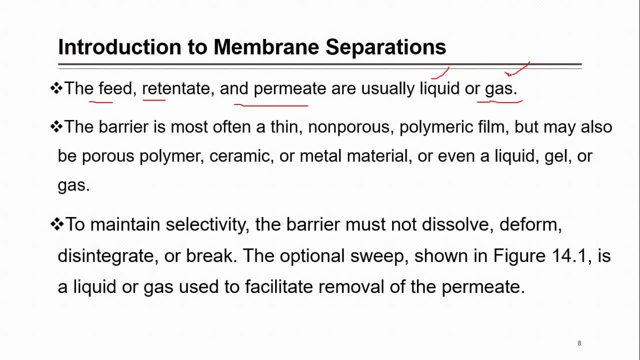 either you pass that gas through this membrane and it allows only hydrocarbon, like CH4 and some other hydrocarbon, to pass through, or this can be somehow the opposite way, that allows only like CO2 and H2S to pass through, and I mean then this gas which is like your. 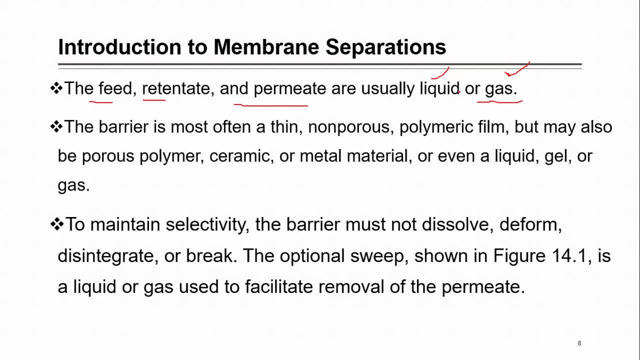 component of like advantage, or you can say which is beneficial to us, So that will just leave as a retentate. so finally, overall, you can say that like these feed, retentate or permeate, all will be usually the liquid or gas inside the system. 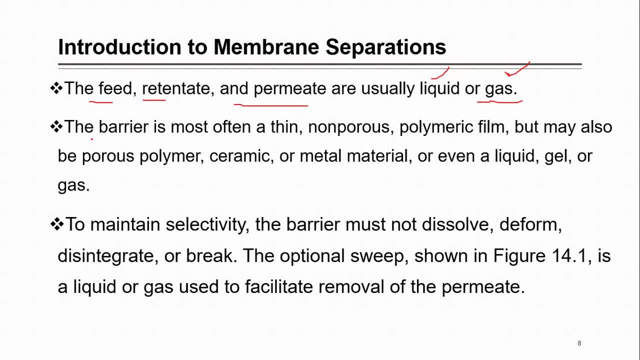 But sometime you can have them as like solid. finally, suppose when you look at reverse osmosis, and in reverse osmosis that is actually technology which use membrane and that is used for purification of water. So in that case, actually, you will see that your solids are rejected, sorry, salts are rejected. 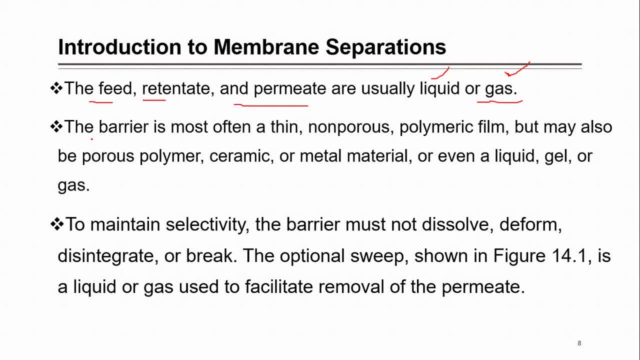 as a solid. So sometime you can have them as a solid, but most of the time you will be looking at all these three mean feed. retentate and permeate are actually liquid or gases, but that is not necessary, as I have given you the example of salts. 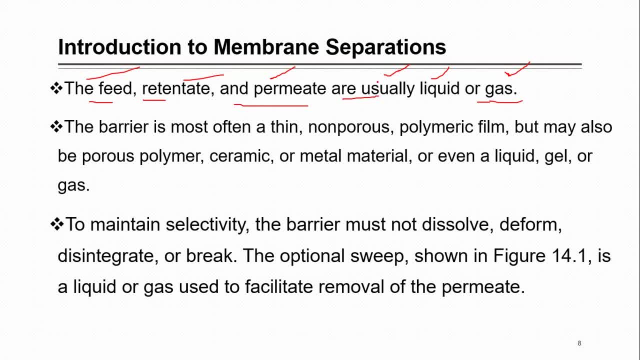 So if salts are rejected at then from the water, actually when concentration will increase their salts concentration. So because you are removing them from the water, and when you are removing the water, you know that they will start crystallizing and they will appear as a solid. 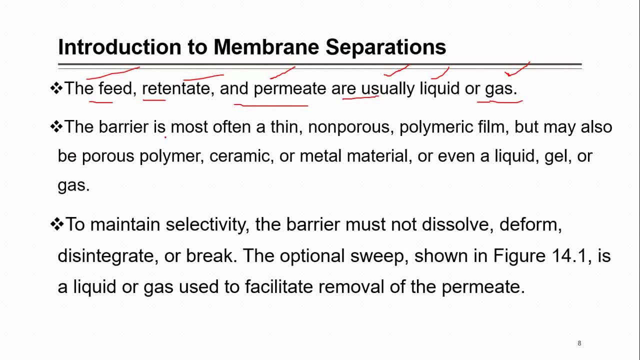 This barrier which is being used as a membrane is often thin, non-porous and polymeric film. I mean when we will talk about the material of these membranes, So you will see that they are commonly, most of those membrane are, most of those are polymeric. 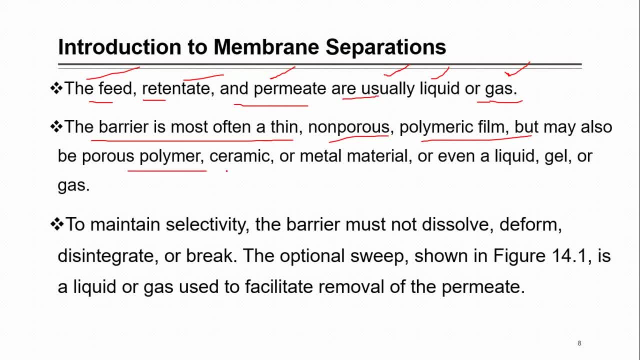 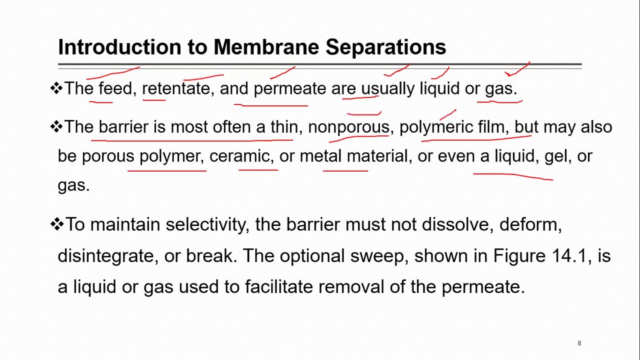 but at the same time they can be all sometime, as I mean like ceramic or metallic material membrane. Even sometime you will see that they can be in the form of liquid gel. So that cannot be also used as a membrane. So they also come in like two categories. like this is based on material of construction. 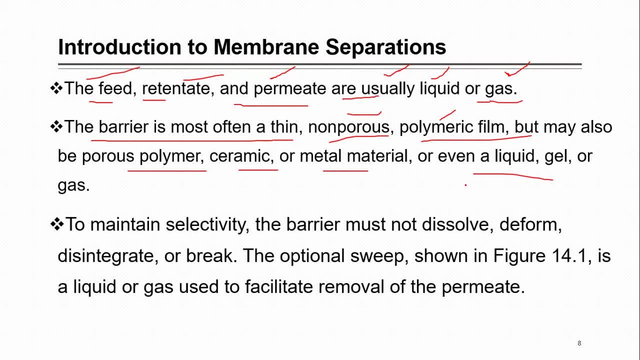 like they can be polymeric, ceramic, metal or even liquid gel, but other based on their- like- porous or non-porous- structure. Some of them can be like non-porous, I mean they do not have any pores, While other are somehow porous- I mean they have pores- and based on when membrane will. 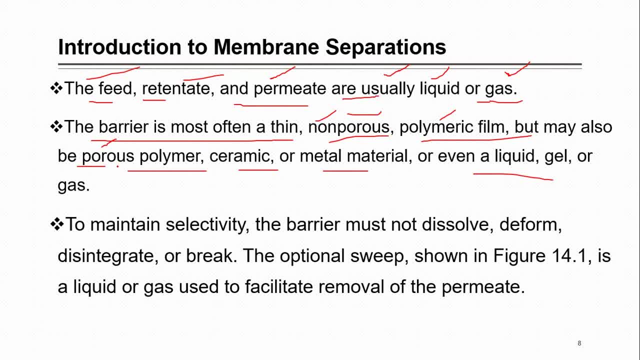 be porous. you know that separation will be mainly based on size separation. I mean, if it is porous and pores will be of some specific size, So they will allow some of the component to pass through, while other will be retained. but as I have told you in the first slide, where we have seen that through one membrane, 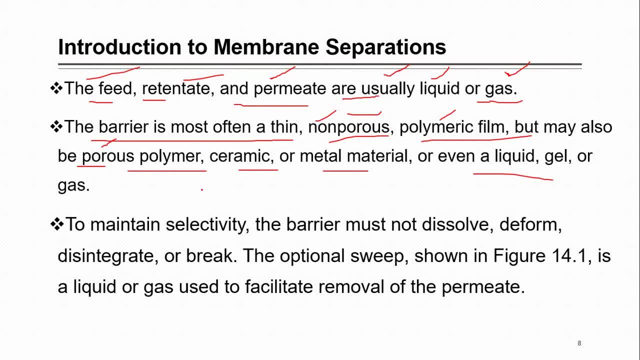 even that membrane is more selective towards large size particles. So there you will see later on, Later on, that actually separation is not taking place based on size. Those membrane are totally non-porous, They did not contain any pores, but overall separation will take place through some other. 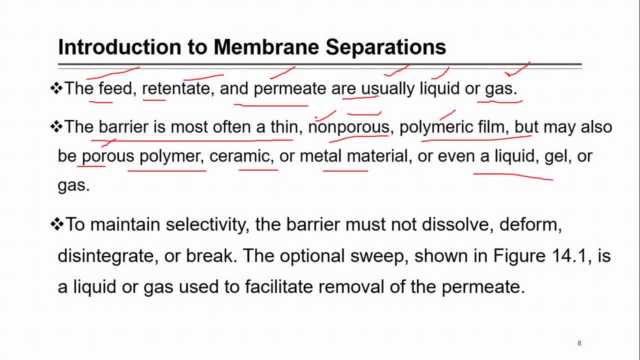 phenomena, which we will, I mean, see that that is something called diffusion. So diffusion through the membrane takes place, non-porous membrane, So through those membrane. actually it is not based on the size, It is based on diffusion. I mean, some component can easily diffuse through that membrane. 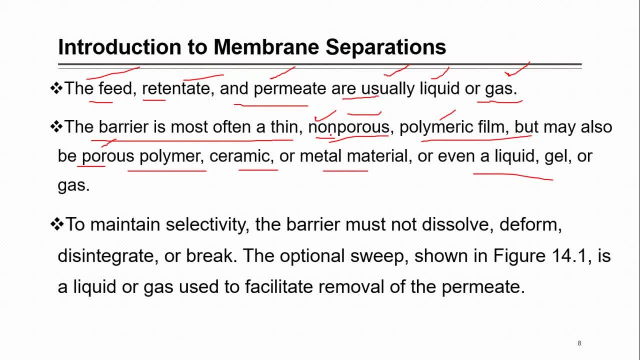 So it is not based on the size, It is based on diffusion. Some of the membrane can pass through that membrane and while other will not pass through. that is not based on size. actually, that is its diffusivity through that membrane material. So next, I mean, when you look at these membrane and we are looking for specific selectivity- 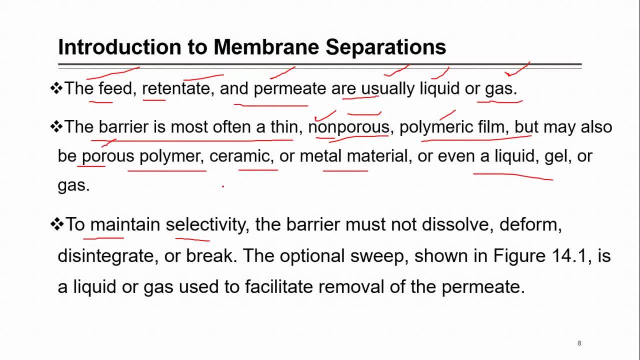 Selectivity means I mean something which we want to selectively remove with the help of the membrane, With the help of this. So to maintain selectively, barrier must not dissolve, deform, disintegrate or break. It means actually, your membrane should be stable. 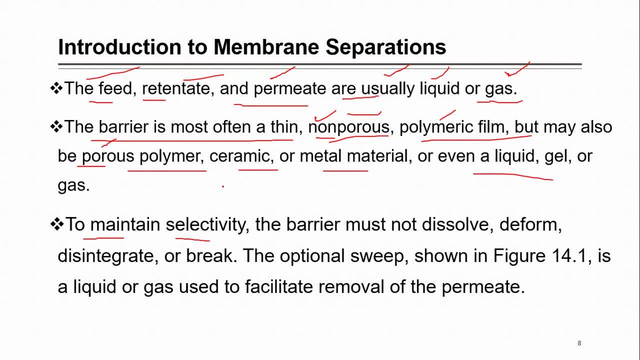 It should not be like a reactive. It should not dissolve inside your feed. I mean it should not break. If it will break, definitely I mean this will not be working properly as well if it dissolve some of its component or remove with the feed. 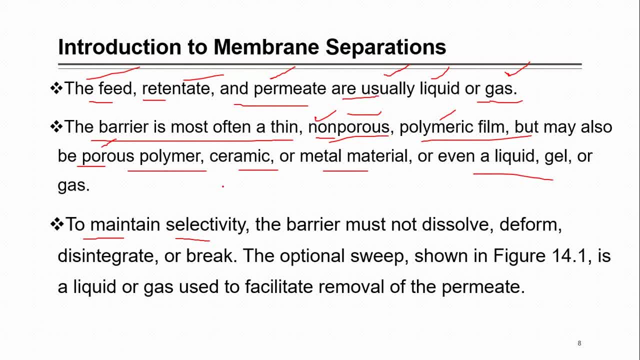 They become part of the feed in the form of retentate or permeate, So that will be actually the damage. So in order to avoid that, mean that membrane: if you want purity, you want good separation, So your membrane should not have like these kind of problems. 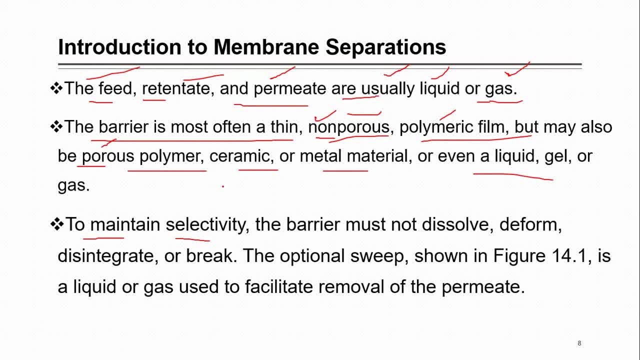 Like optional sweep which we have seen somewhere inside the figure which I have told you that this is from your text books. So optional sweep we were using that was being used to facilitate removal of the permeate. So I mean we have seen at this. at that time I have told you that you can just pass some. 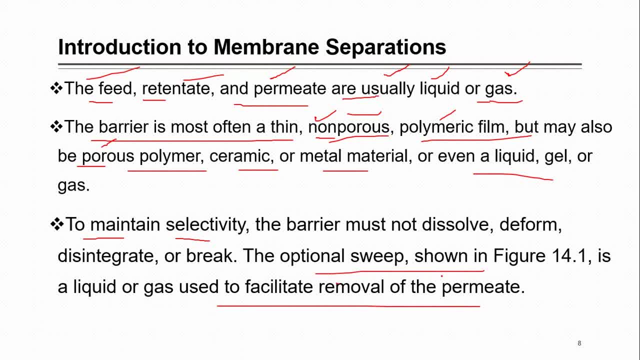 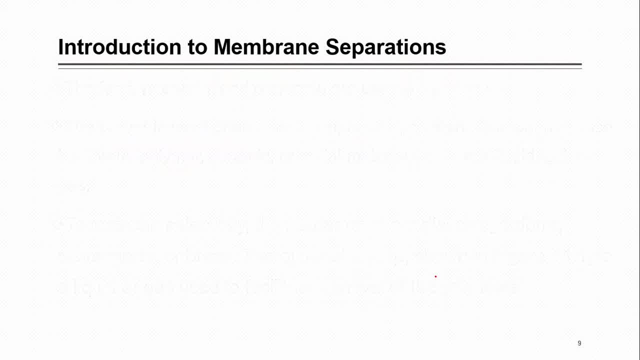 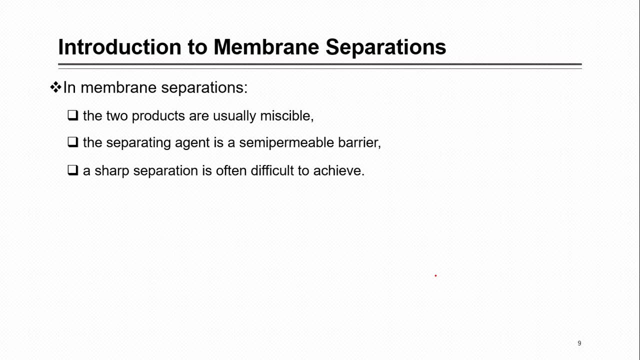 liquid or gas through this system at the high pressure So that it will push the permeate which is accumulated inside system that can be easily removed. So, overall, when you look at this membrane separation, actually I mean the products which 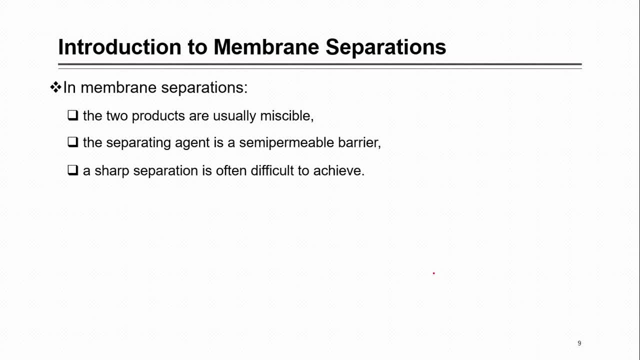 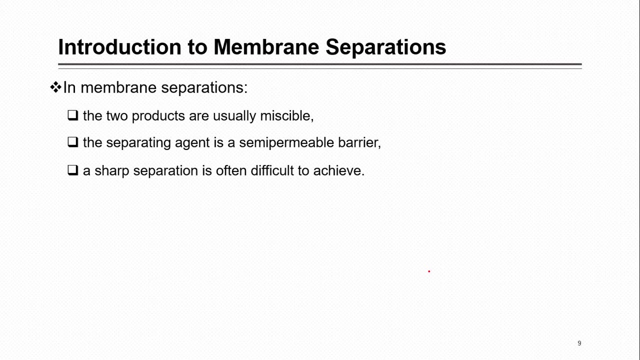 you are getting here from the feed. they are usually miscible. like what does this mean? I mean they are usually soluble. They are, I mean, in the form of one phase, For example. I mean here we have talked about one thing like gas, natural gas and natural. 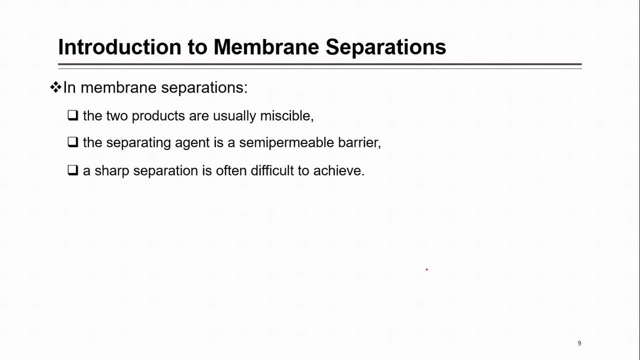 and natural gases in the form of like mixture of gases, So they all are miscible with each other. they will be, they will appear in the form of one phase actually. I mean you cannot distinguish between them. So when you will pass through this membrane, the products which you are getting, they 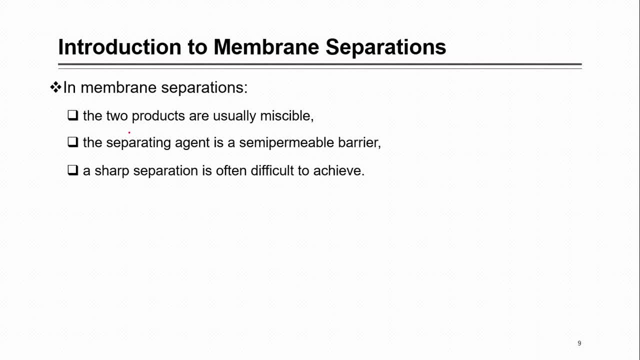 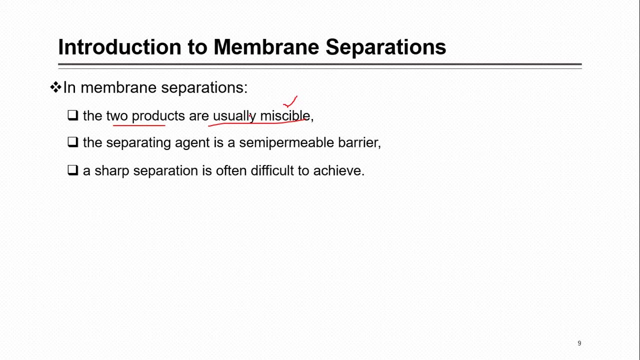 are now separated, like one is permeate and other is retentate, But initially they were the two products which you are getting in the form of permeate and retentate. they were miscible. I mean when they are miscible. So the this the problem. actually, we have to separate them, So that can. 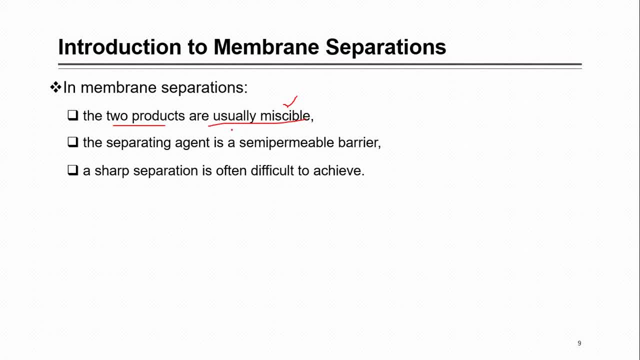 be separated with the help of anything, but in membrane- like you when you are looking at this, they are usually miscible with each other. So they can be separated with this membrane into two component, and then they will be like just separated out, They will become somehow we can. 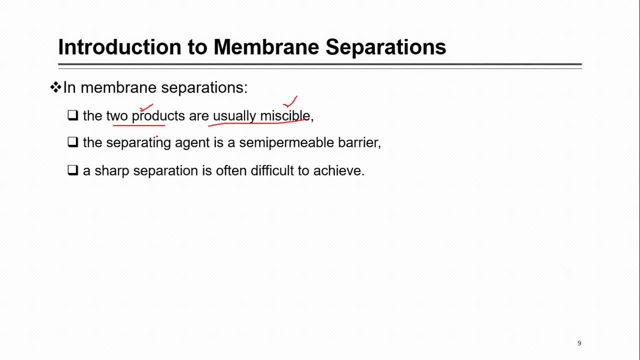 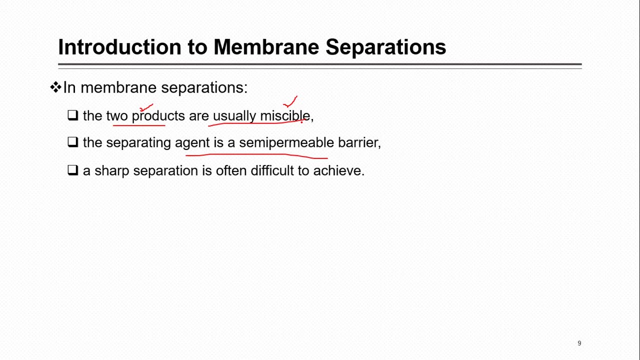 say immiscible, not immiscible in terms of this separation. actually they will get separated. the separating agent here is semipermeable barrier. actually, when you just compare this technique with the other techniques which you have talked about, So you can see that separating. 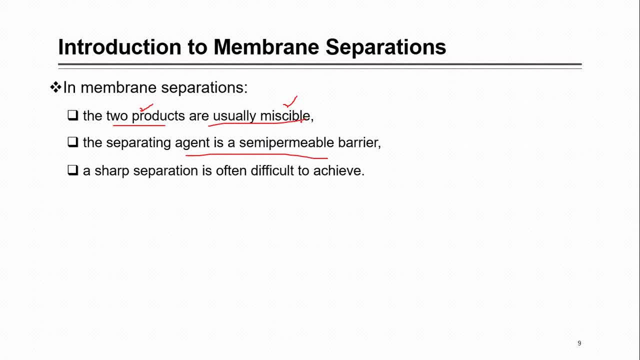 agent. always we look at some separating agent, like if you are looking at phase creation separation, So, in which the phase is created with the help of, like, maybe temperature or pressure, as we have seen- some cold ring. So when you open the lid, So what happens? actually you are reducing the pressure. So 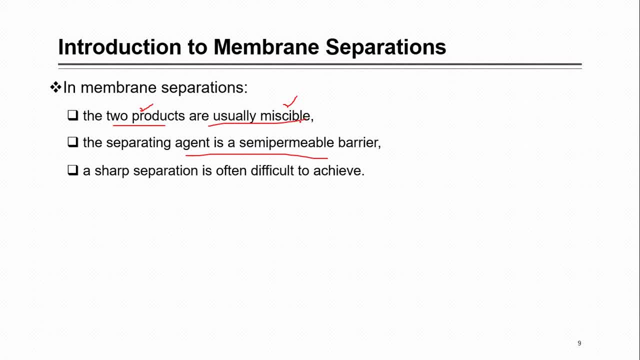 here your pressure is the separating agent as well. if in distillation you heat the feed, So there the heat, the temperature, is your separating agent. In liquid-liquid extraction you have seen that our externally introduced liquid was the separating agent. Inside absorption, you remember. 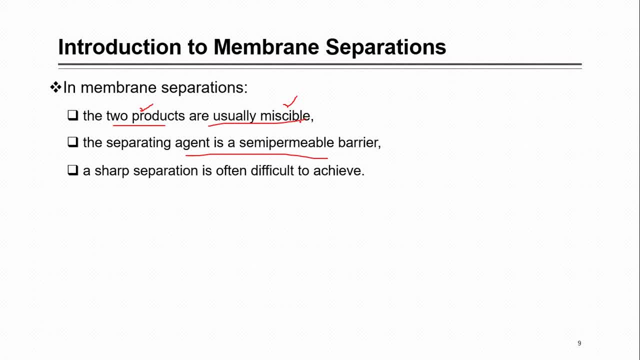 that some externally introduced solvent which was absorbing some of the component through the- I mean- feed. that was separating agent. So here actually separating agent is some semipermeable barrier and that is membrane. So here in membrane separation, sharp separation is often difficult. 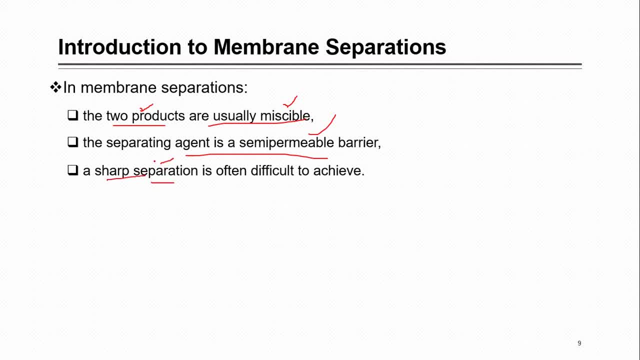 sharp separation, as we have seen. sharp separation mean, as you have seen that, 100 percent separation. I mean that is a bit difficult because membrane will allow some of the components- other component will also- to pass through, which we do not want actually. I mean they are not like 100 percent. 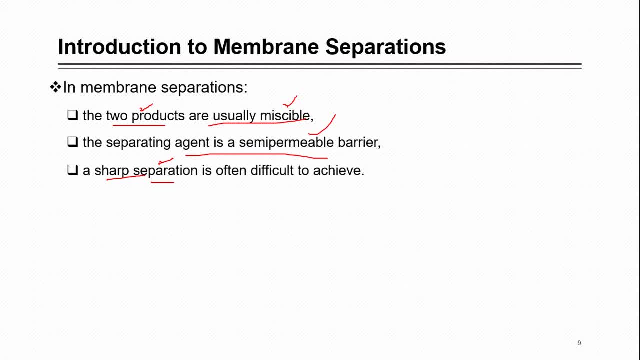 removing, and this problem exist in more or less all techniques. actually, you cannot get 100 percent separation, or if you are looking for very high purity or such stuff, may you go for more than one stages, as we also talked about. this, like in liquid-liquid extraction, as well mean in absorption. 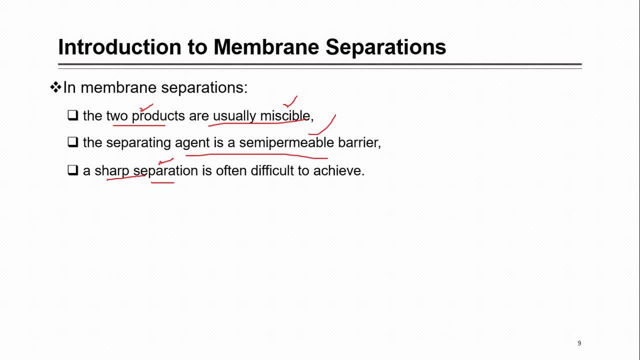 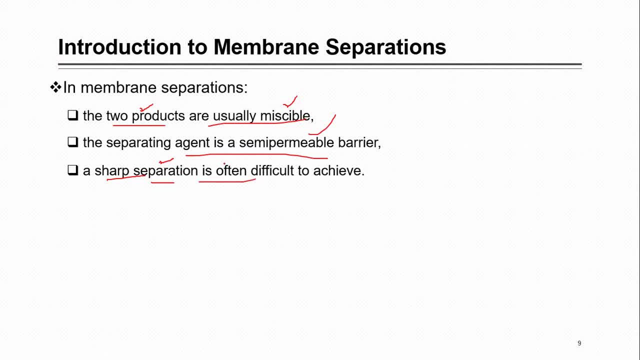 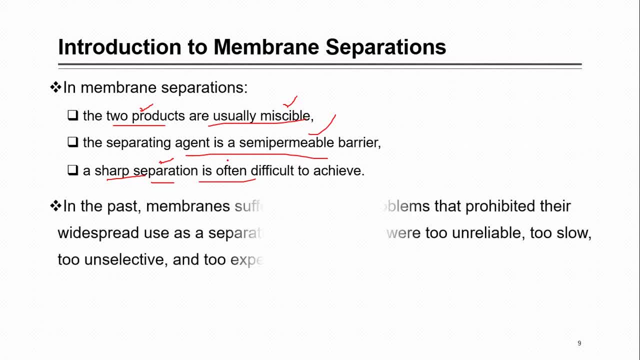 one module to pass your feed, one module to pass your feed through this, that you can get better through this, that you can get better through this, that you can get better separation. So, when we look at the separation, So when we look at the 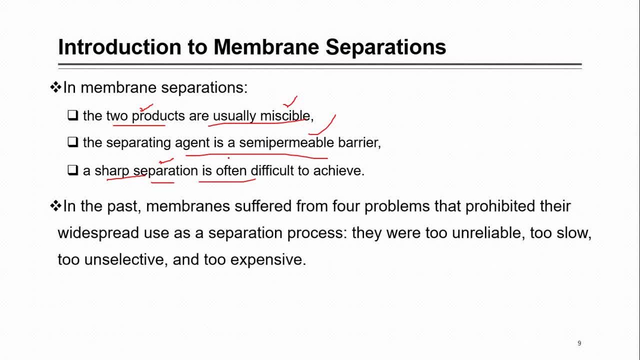 separation. So, when we look at the membranes, actually they are being used in membranes. actually they are being used in membranes. actually they are being used in industries. now many industries are using industries. now many industries are using industries. now many industries are using these membranes on commercial scale. mean, 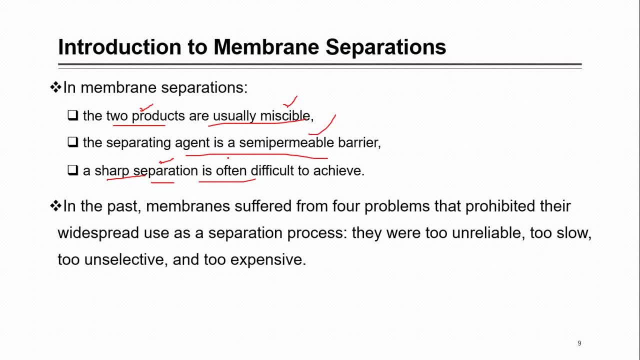 these membranes on commercial scale mean these membranes on commercial scale mean they are being used. But if we look at, they are being used, But if we look at they are being used, But if we look at the past actually mean membrane has. the past actually mean membrane has. 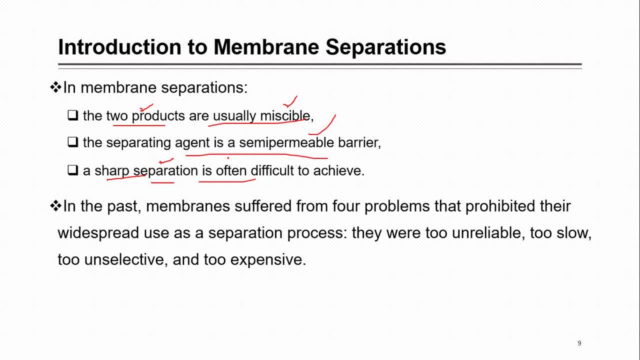 the past actually mean membrane has suffered from various problem and they suffered from various problem and they suffered from various problem and they were actually four common problems, which were actually four common problems, which were actually four common problems, which membrane were facing and those include membrane were facing and those include 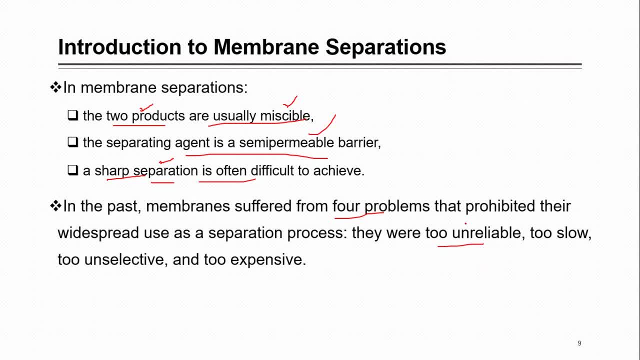 membrane were facing and those include: actually they were too unreliable to actually they were too unreliable to actually they were too unreliable to unreliable mean they were not giving very unreliable mean, they were not giving very unreliable mean, they were not giving very good separation. sometimes they are good separation, sometimes they are. 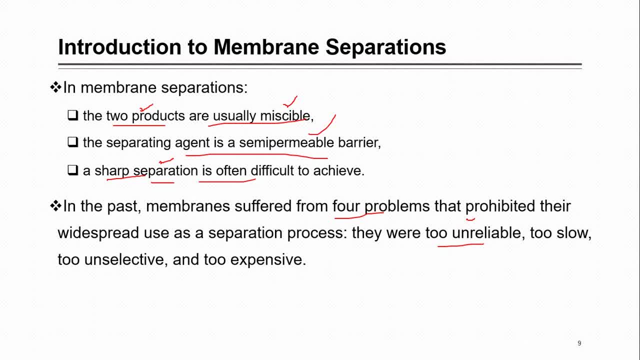 good separation. sometimes they are performing well, sometimes they are not as performing well, sometimes they are not as performing well, sometimes they are not as well. they have some problems like they. well, they have some problems like they. well, they have some problems like they were too slow. because this is the 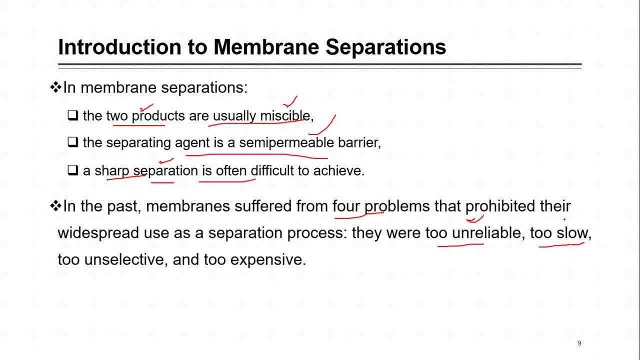 were too slow because this is the were too slow because this is the barrier, as we have seen, that if membrane barrier, as we have seen that, if membrane barrier, as we have seen that if membrane is sometimes porous, sometimes non porous, is sometimes porous, sometimes non porous, is sometimes porous, sometimes non porous, membrane can be used. so, if you are using 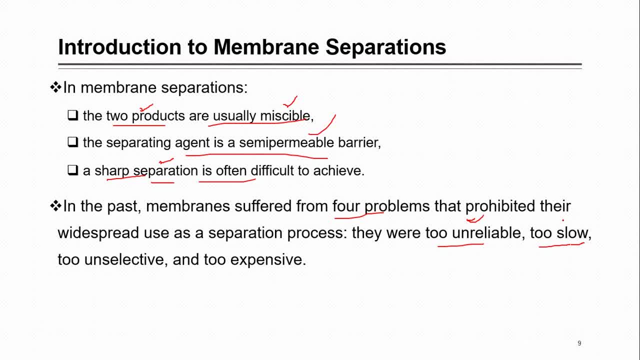 membrane can be used. so if you are using, membrane can be used. so if you are using, like some of non porous definitely mean like some of non porous definitely mean like some of non porous definitely mean there are no pores and now you have to. there are no pores and now you have to. 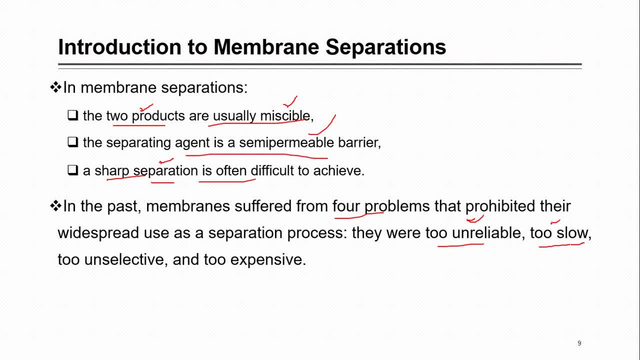 there are no pores. and now you have to separate two components, so it works. separate two components, so it works. separate two components, so it works. somehow like slowly as well, you can have. somehow like slowly as well, you can have. somehow like slowly as well, you can have, like they are, to select unselective. 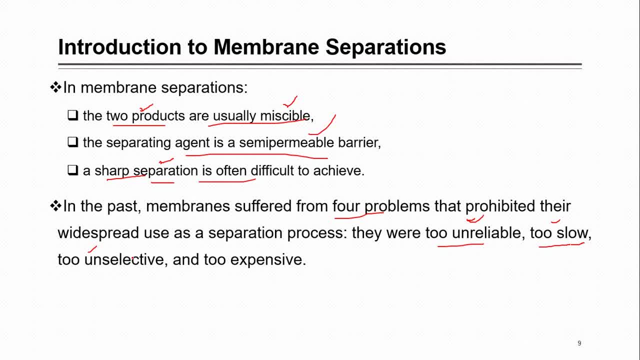 like they are to select unselective. like they are to select unselective because when, if we want to separate the because, when, if we want to separate the because, when, if we want to separate the feed, suppose we were separating natural feed. suppose we were separating natural. 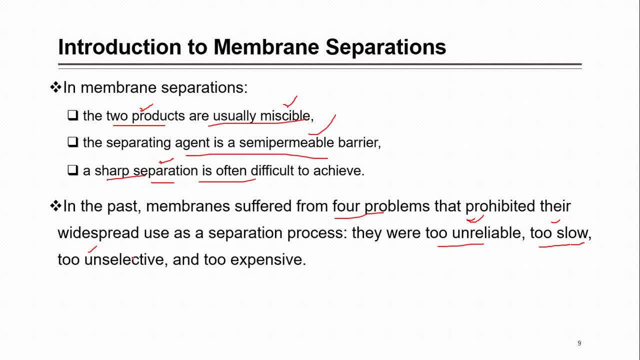 feed. suppose we were separating natural gas CH4 from the impurity co2 Rh2s. so it gas CH4 from the impurity co2 Rh2s. so it gas CH4 from the impurity co2 Rh2s. so it is like it allows along with natural. 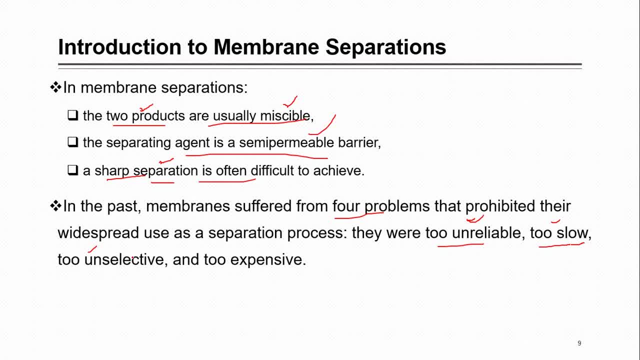 is like it allows along with natural is like it allows along with natural gas, CH4 and other hydrocarbon. it allows gas CH4 and other hydrocarbon. it allows gas CH4 and other hydrocarbon. it allows also co2 plus H2s to pass through or. 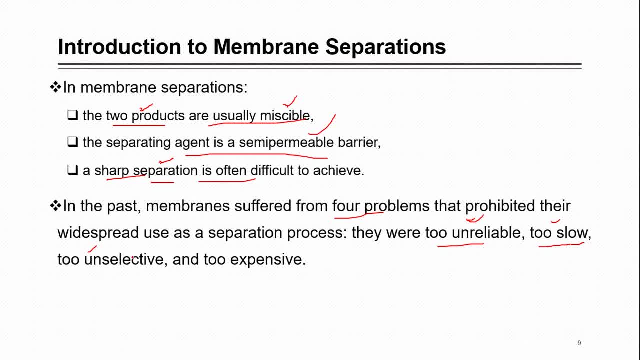 also co2 plus H2s to pass through, or also co2 plus H2s to pass through, or, for example, you can take the example of, for example, you can take the example of, for example, you can take the example of air, if we want to separate it into. 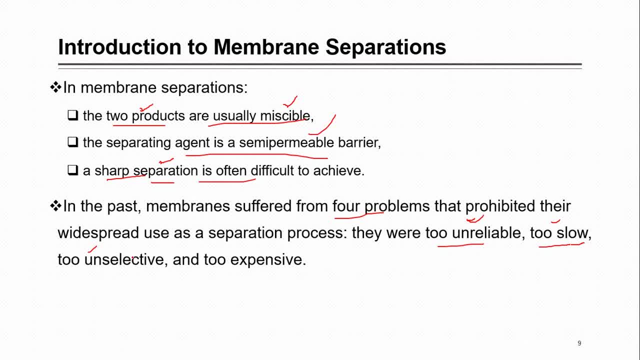 air, if we want to separate it into air, if we want to separate it into oxygen and nitrogen. so I mean, if you oxygen and nitrogen, so I mean if you oxygen and nitrogen, so I mean if you allow air to pass through this membrane, allow air to pass through this membrane. 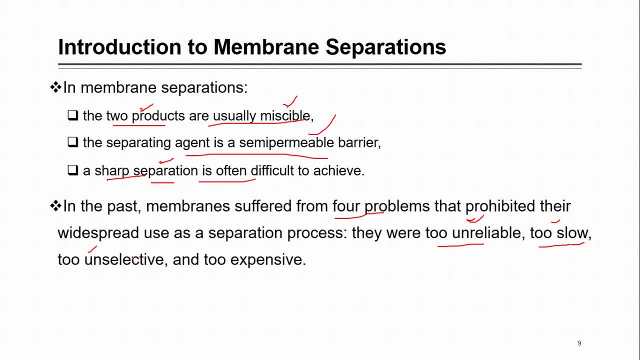 allow air to pass through this membrane. and suppose we just consider that this, and suppose we just consider that this, and suppose we just consider that this is selective towards oxygen, selective is selective towards oxygen, selective is selective towards oxygen. selective toward oxygen mean it allows oxygen to. toward oxygen mean it allows oxygen to. 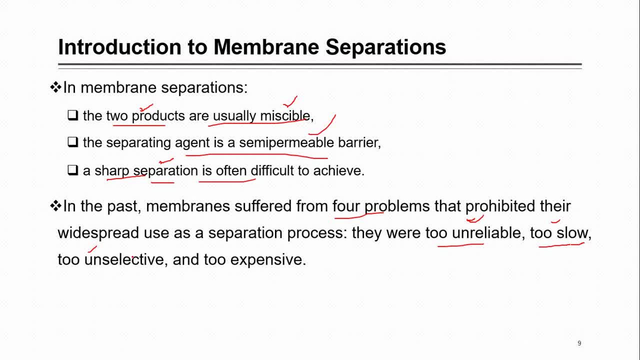 toward oxygen, mean it allows oxygen to pass through mainly, but with this, some pass through mainly, but with this, some pass through mainly, but with this some nitrogen will also pass through. this nitrogen will also pass through. this nitrogen will also pass through. this other component which we were looking to. 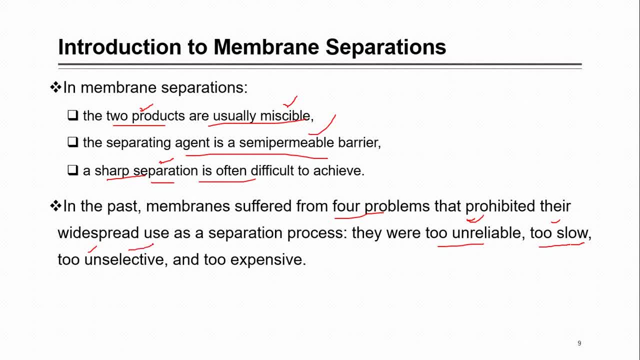 other component which we were looking to, other component which we were looking to be separated that also pass through. this be separated. that also pass through. this be separated, that also pass through this. so this was a problem of on selectivity. so this was a problem of on selectivity. 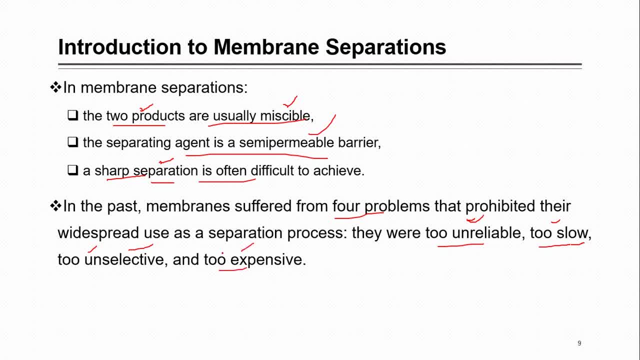 so this was a problem of on selectivity and they were also too expensive. mean it and they were also too expensive. mean it and they were also too expensive. mean it is expensive to build the system. so when is expensive to build the system? so when is expensive to build the system? so when you have compared these main membranes, 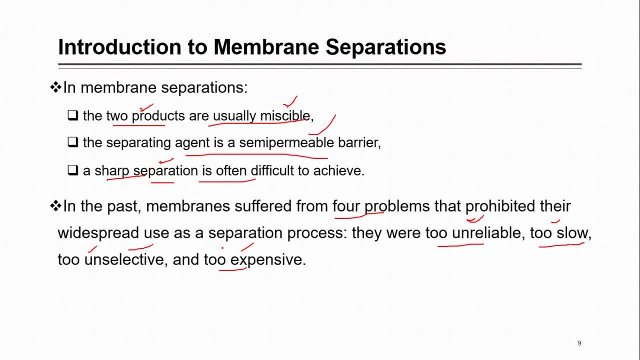 you have compared these main membranes. you have compared these main membranes with the other technology, the existing with the other technology, the existing with the other technology. the existing system like distillation, absorption and system like distillation, absorption and system like distillation, absorption and liquid extraction are some other. 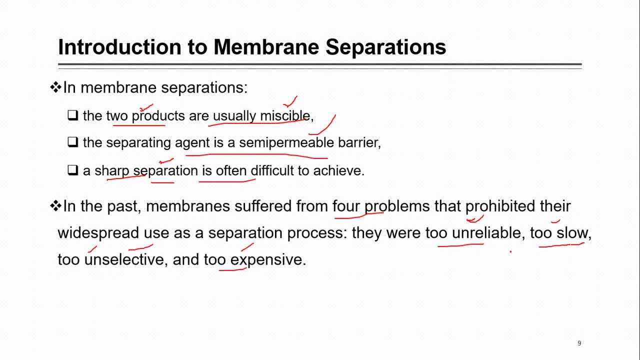 liquid extraction are some other. liquid extraction are some other techniques. so, compared to them, these four techniques. so compared to them, these four techniques. so compared to them, these four problems were present in membranes, but problems were present in membranes, but problems were present in membranes, but with the passage of time, in these, 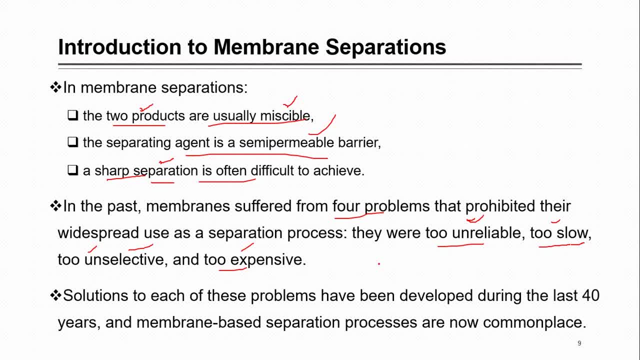 with the passage of time in these, with the passage of time in these, problem has been solved and in the last problem has been solved. and in the last problem has been solved and in the last 40 years, more or less, you can see I, 40 years, more or less, you can see I. 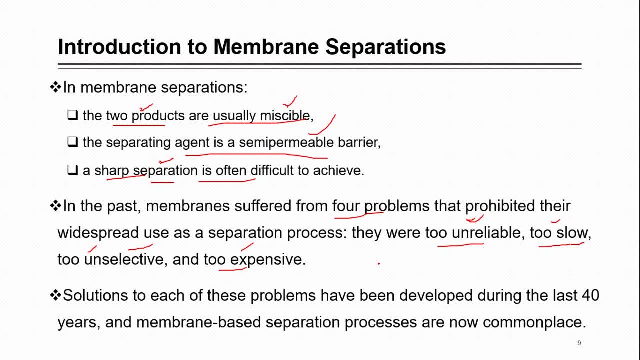 40 years, more or less. you can see, I think your book refer half a century, so think your book refer half a century. so think your book refer half a century. so based on that, actually the membranes, based on that, actually the membranes, based on that, actually the membranes have been developed and 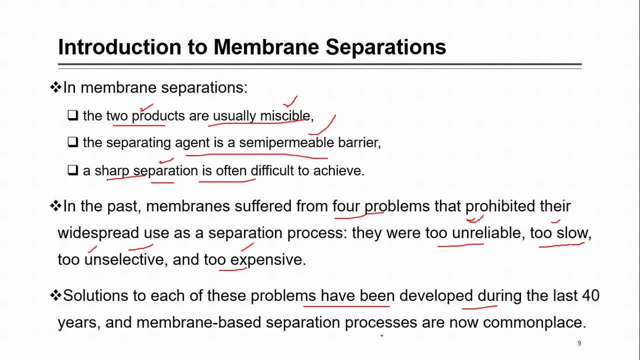 have been developed and have been developed, and their performance has become better. so they. their performance has become better, so they. their performance has become better. so they are being commonly used in. the are being commonly used in. the are being commonly used in the industries now. so here is a brief. 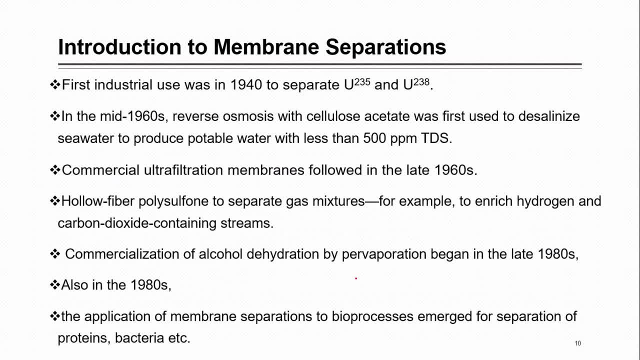 industries now. so here is a brief industries now. so here is a brief history of the membranes. so when you history of the membranes, so when you history of the membranes, so when you look at the membrane so where they have, look at the membrane so where they have, 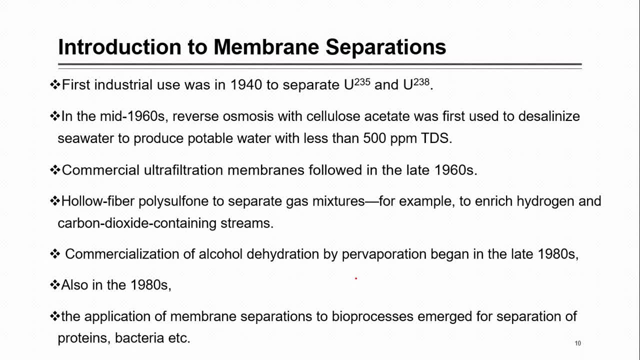 look at the membrane so where they have been used and when they have been used been used and when they have been used been used and when they have been used so you can see their first industrial use. so you can see their first industrial use. so you can see their first industrial use of the membrane was in like 1940 and 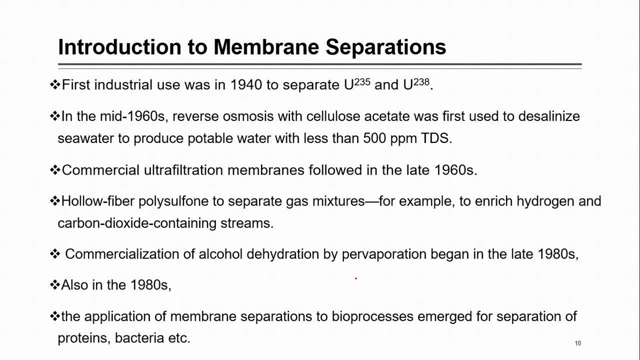 of the membrane was in like 1940 and of the membrane was in like 1940 and that was used for separation of uranium. that was used for separation of uranium. that was used for separation of uranium components. that was in the form of components, that was in the form of. 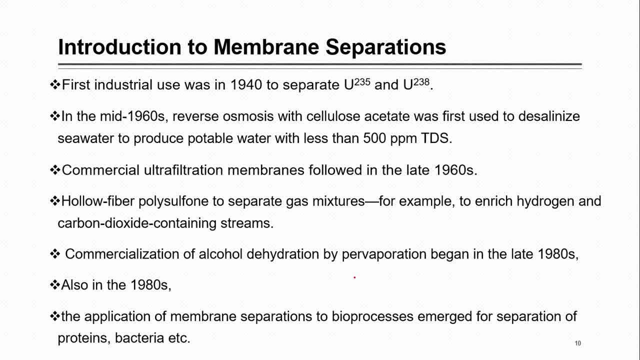 components that was in the form of uranium fluoride, I think, and you have uranium fluoride, I think, and you have uranium fluoride, I think, and you have separated two isotopes of uranium, separated two isotopes of uranium, separated two isotopes of uranium through this. so here you can see this. 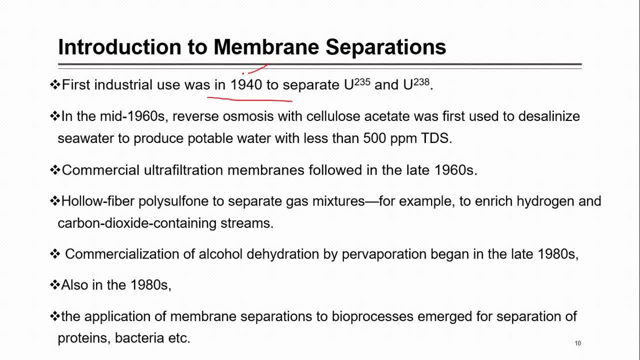 through this, so here you can see this, through this, so here you can see this: 1940, what is important about this year? so, if you remember, this is the time of, so, if you remember this is the time of, so, if you remember, this is the time of World War two and at that time, mostly, 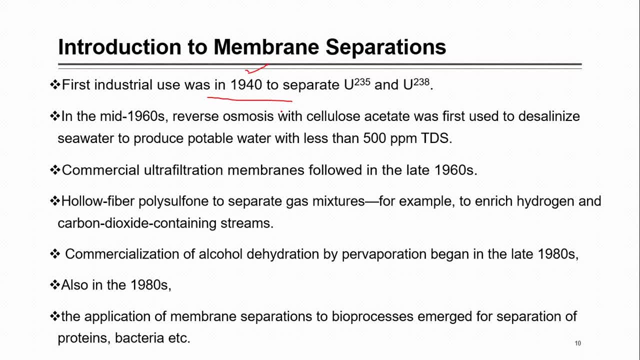 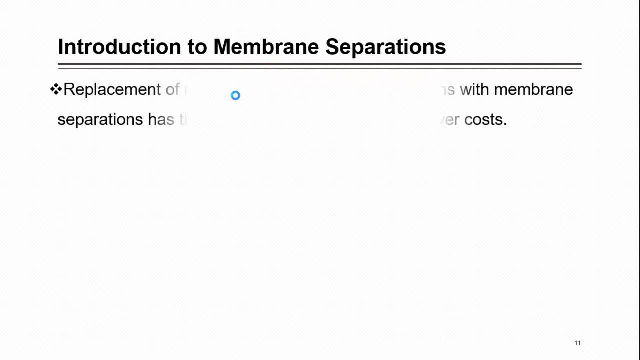 World War two and at that time mostly World War two, and at that time mostly you will look here, there is, you will look here, there is, you will look here. there is also another means here, in which actually also another means here, in which actually also another means here in which actually the most of somehow development took. 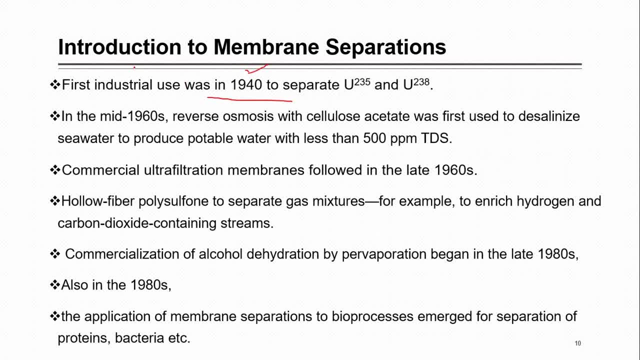 the most of somehow development took the most of somehow development took place. so in that time, this industrial place, so in that time, this industrial place, so in that time, this industrial use of this membrane took place and you use of this membrane took place, and you use of this membrane took place and you have separated uranium isotopes with the. 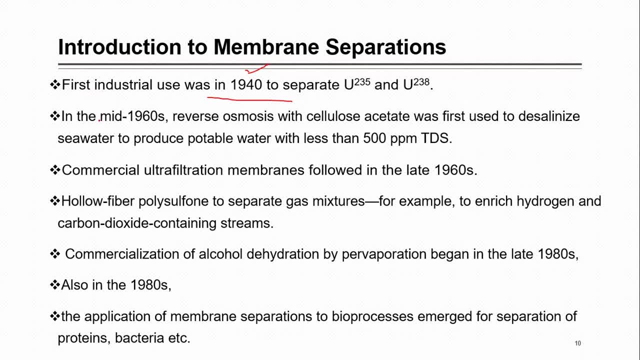 have separated uranium isotopes with the have separated uranium isotopes with the help of membrane. so that was first help of membrane. so that was first help of membrane. so that was first industrial use of membrane and then like industrial use of membrane and then like industrial use of membrane and then, like in mid 1960, reverse osmosis with the. 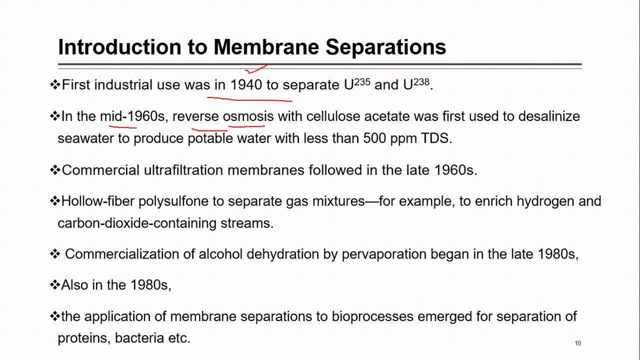 in mid 1960. reverse osmosis with the in mid 1960. reverse osmosis with the cellulose acetone- I mean reverse osmosis- is one of the membrane separation technique which we have to discuss in detail. So in that you have used cellulose acetate membrane, Now cellulose acetate is 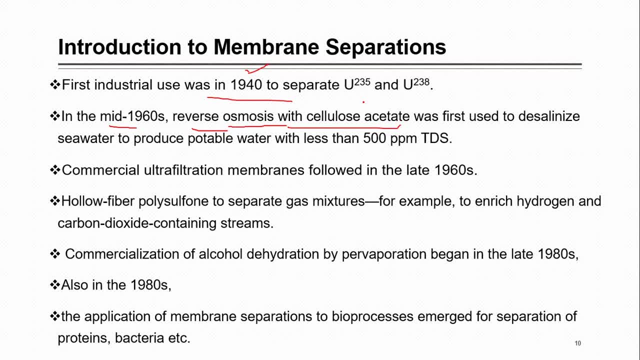 actually material of construction of those membrane. Reverse osmosis is the phenomena in which you have used cellulose acetate membrane, and they were used first time in the mid 1960. They were used for purification of sea water. So it becomes available or means suitable. 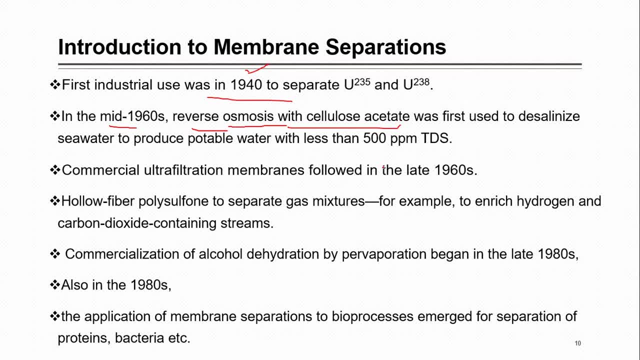 for drinking purpose, and the first time- here I mean from this sea water solids were reduced to like 500 ppm. TDS means total dissolved solids. So they were reduced to less than 500 ppm and with the help of this, when they are less than 500, usually this water is drinkable. 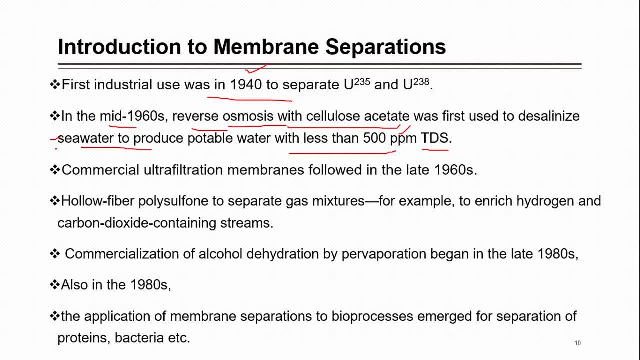 But actually So in seawater. if you look at the seawater, so that contains very high amount of these total dissolved solid. they are somehow in the range of, I think, 30,000 ppm to 50,000 ppm mostly. So they are reduced to how you can see here that now at these membrane, reduced those from. 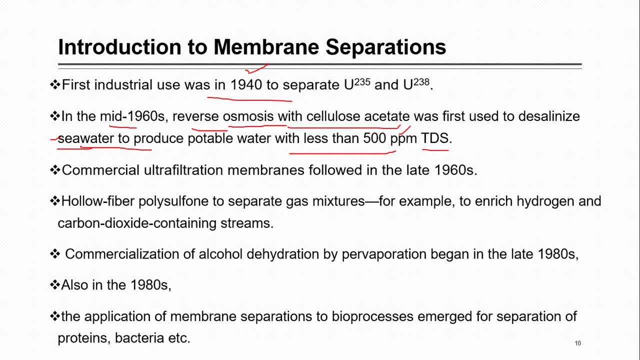 maybe 30,000 or somehow mean they, this is very big value, so to say 500 ppm. so this was the first industrial use of cellulose acetate for cleaning of water, seawater. Then there is one type of membrane. ultrafiltration like this is also one type: reverse osmosis. 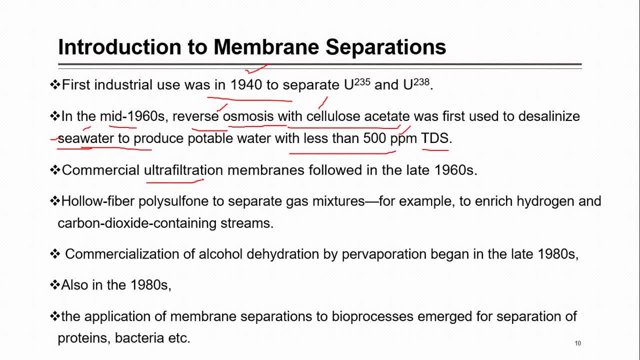 so ultrafiltration, this is based on actually their size, pore size ultrafiltration. then you will hear: I think see something called microfiltration somewhere may be mentioned, or that is also one type. So ultrafiltration was also followed in like 1960 after this. 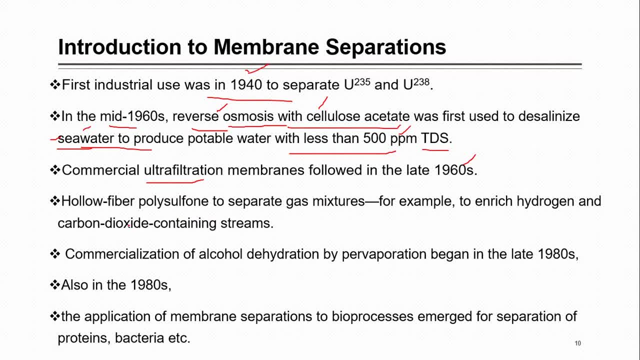 This reverse osmosis, somehow that was also used on industrial scale mean that membrane was also used. Then there were hollow fiber, polysulfone, membrane polysulfone, now again one of the polymer mean. with the help of that, some these hollow fiber membranes were formed and they were used for 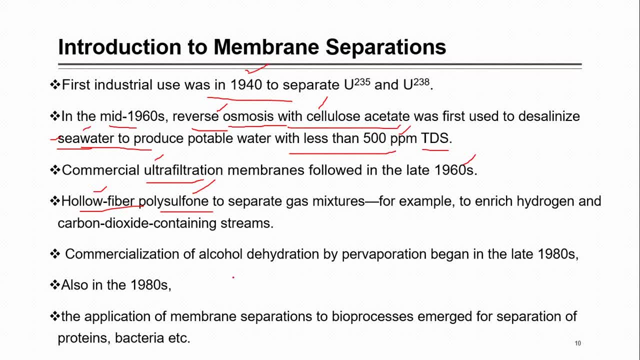 separating the gas mixture first time- and that gas mixture was actually hydrogen and CO2 mixture- And this membrane were used for their enriching or their mean separation And then their mean commercial commercialization of alcohol dehydration were by pervaporation. A pervaporation is one of the technique in membrane. again, we will talk about this in. 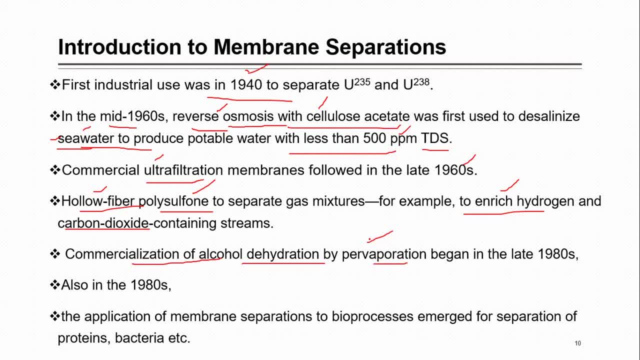 detail later on. this is the part of mean, this study, this chapter, So in that, actually also here, Actually, what we do, alcohol dehydration: what does this mean? like removal of water from alcohol, So through pervaporation. So overall, you can see, you will see, in this technique actually we have a membrane as well. 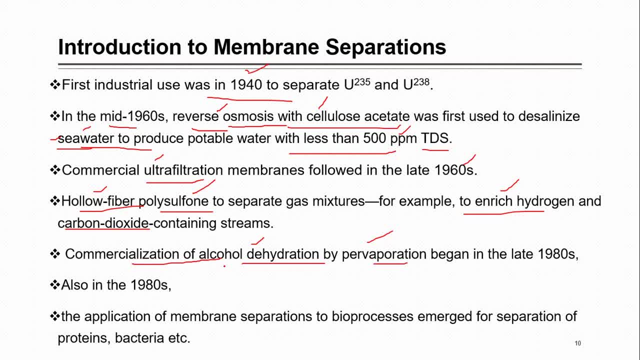 here vaporization is taking place. So based on this, we have a pervaporation, named it as pervaporation, So dehydration from alcohol, we remove the water. So through this technique- and that took place in like late 1980s, Also in 1980s- 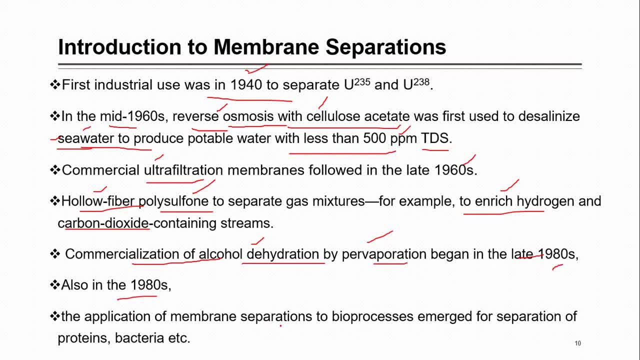 So in 1980s, So in 1980s, the application of membrane separation to bioprocesses took place And if you will look at the literature, I mean in this era also a lot of development took place, and I think it was the time of like Arab-Israel war, I think, and in that time many 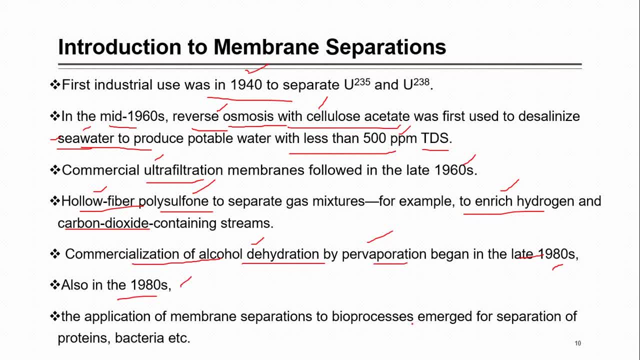 developments took place. So, like they were also used for bioprocesses and in bioprocessing, actually, what you do? you separate the some high proteins. They were also used for bioprocesses And in bioprocessing, actually, what you do? you separate the some high proteins? 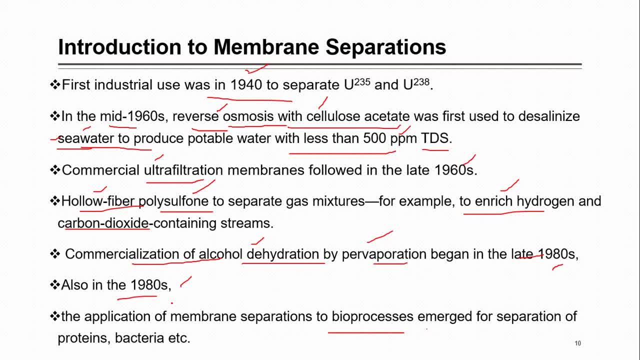 They were also used for bioprocesses, And in bioprocesses, actually, what you do you separate the some high proteins? And in bioprocesses, actually what you do, you separate the some high proteins. They were also used for the separation, or main separation, of bacteria and yeast- somehow. 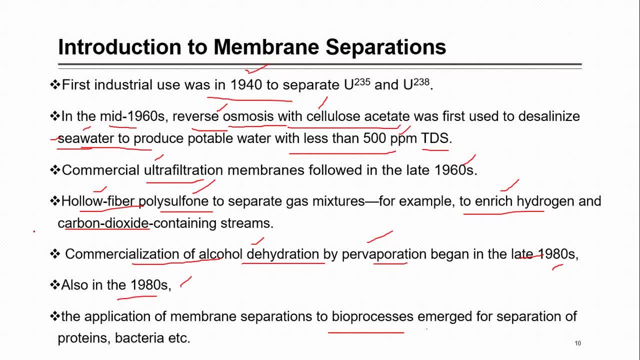 So this is just brief introduction about membrane separation in terms of like their development with the passage of time. So, as I said, here there is some terminology like ultrafiltration, there is pervaporation, there is reverse osmosis and I was talking about also micro filtration. 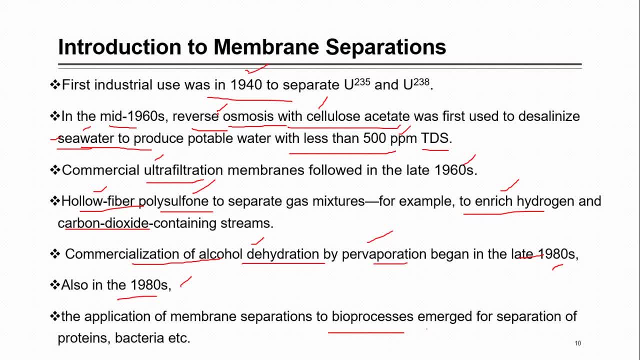 So do not worry about these. These we have to define later on. I mean just because this is introductory lecture and some of the terminologies will not be clear to you, but we will talk about them in detail, actually, later on. So but just 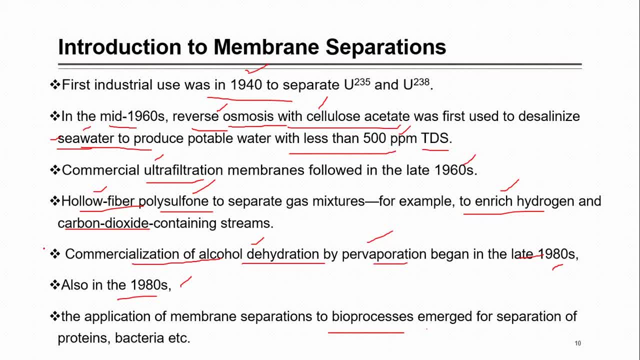 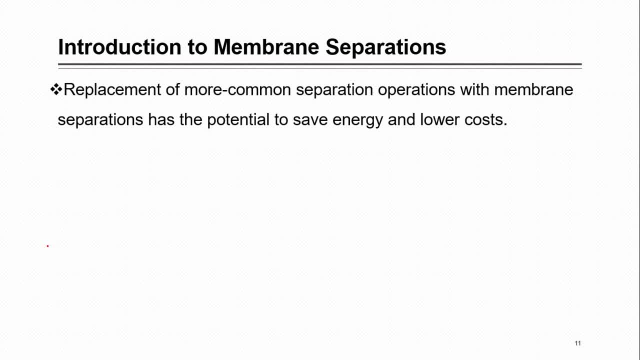 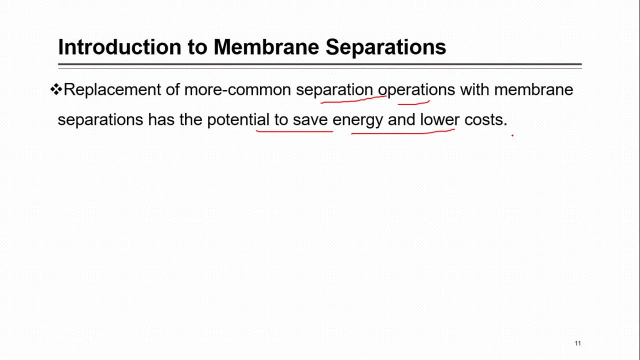 from here. remember that they were developed, you know that with the passage of time. So if we want to replace other- I mean separation operation with the membrane, So they that can be beneficial to save energy as well as with, in terms of cost, actually one slide back. 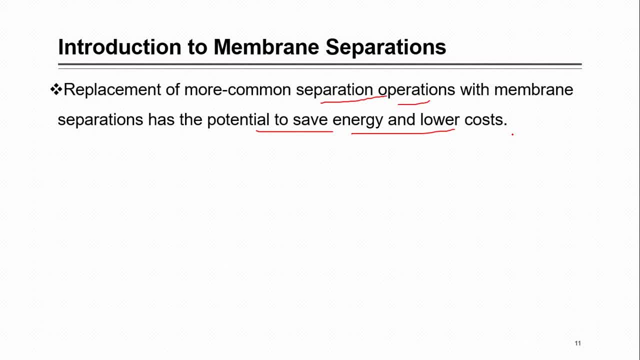 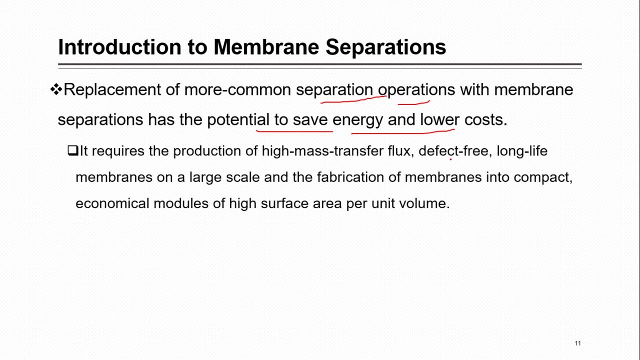 we talked about this- that in the initial stages membrane were not like reliable. they were slow, they were expensive, but with the passage of time many improvements has taken place As well. their price has reduced and they will. they have become more reliable. due to this, they are being used on industrial scale, but still I mean there are some problem, like they. 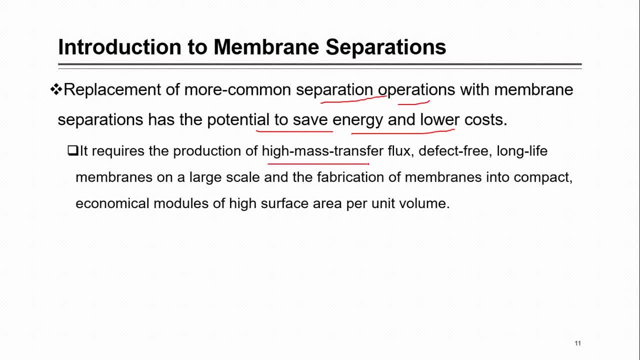 require high mass transfer flux. Mass transfer flux mean actually, as we said, that we have to pass components through the membrane, So they should provide good flux based on selectivity, like they should be selective for one component, and they should allow- I mean- good mass transfer. 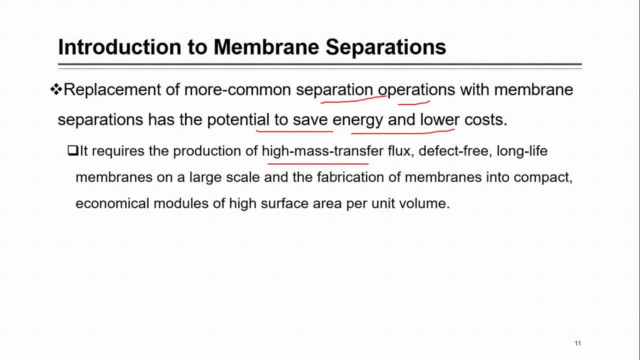 of that component through the membrane As well. they should be defect free and long life membrane on the large scale. I mean these are some requirements like they should be defect free, they should be, they should have long life, because if you will study the membrane you will see that most of the time membrane 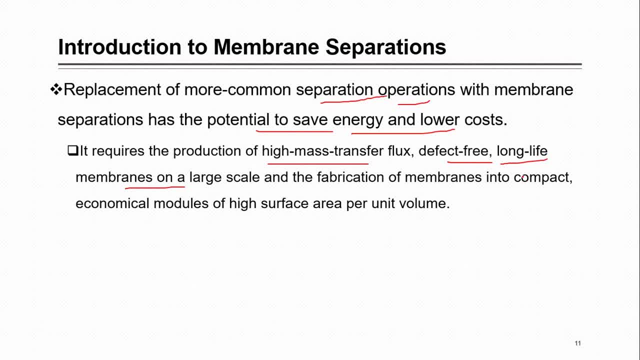 still in the industries you have to replace the membrane. may be after 1 or 2 year at some time, it depends on the application. may be after few months. So that is the problem if you are. I mean just replacing membrane after every few years. 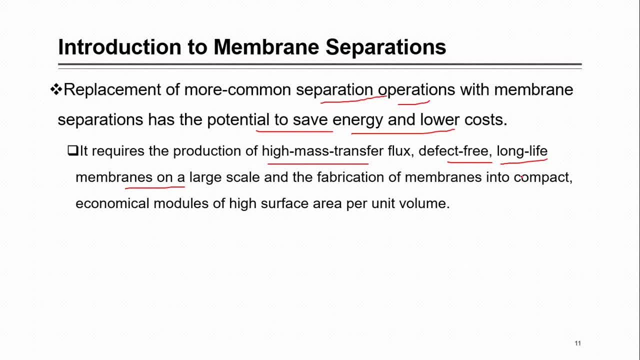 every few months, So that will become expensive process. So if we can design such membranes which provide good flex and they are also long lasting, So that can be good replacement of other separation processes on large scale As well. the other requirement is like we should have, I mean build this membrane module into 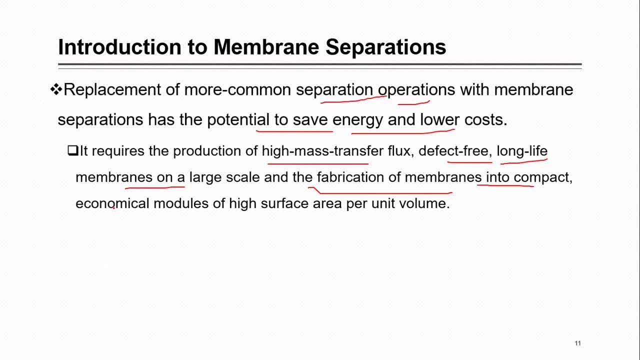 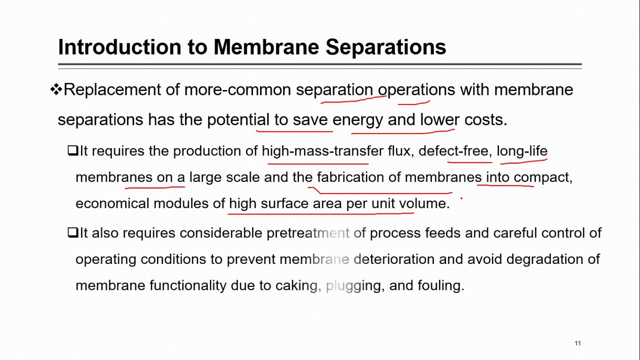 the compact and their fabrication should be compact. Compact mean actually they should have high surface area per unit work So they occupy less space and overall their construction is easy. So these then can be. it can be advantageous as compared to the other separation technique which are commonly 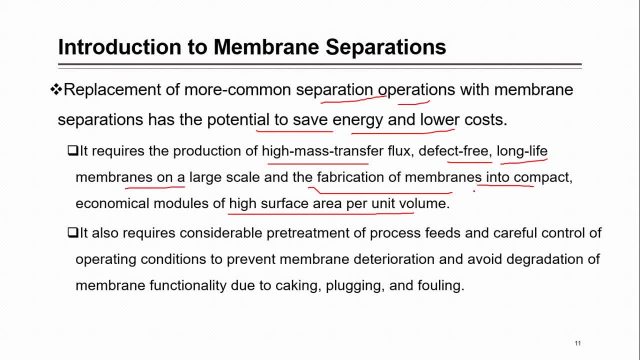 used in the industries. At the same time, this replacement also requires something considerable: pretreatment of the process feed. What does this mean? actually, when you pass some components through the membrane, you are looking for the separation through the membrane. sometime, cake- means one layer of the cake- take place on the surface of membrane. 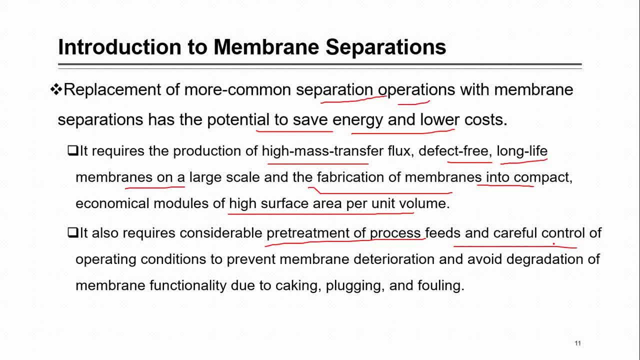 I can give you the example here. like in the lab, like we have seen, lab scale separation through the funnel mean you are passing your solution And that is separated into like mean solid and the liquid, So the solid which is left over on the surface of filter. what? 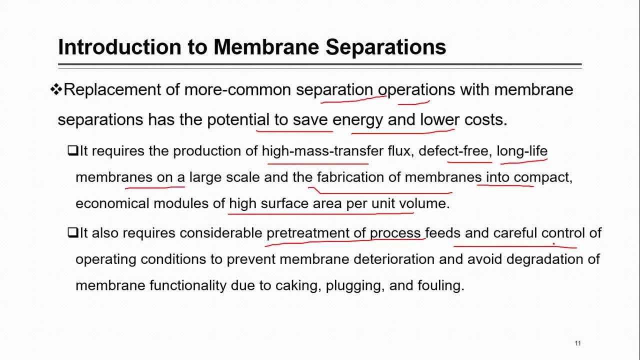 you call it cake. those crystals are Media travel, evolution. This is called Asylt, & Anyways, Here, complex layer communication is a known named as cake actually. So that same can take place on the surface of membrane when 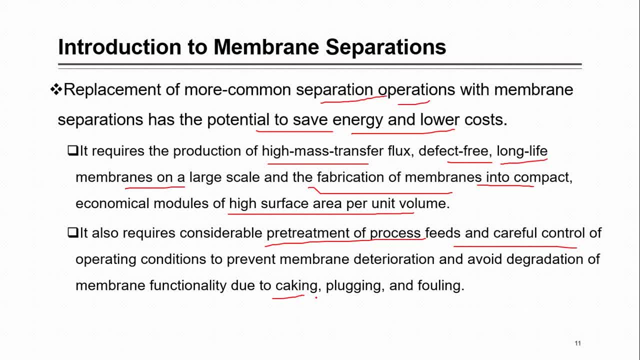 you are passing some of those component through the membrane. So, if like, look at the water containing salts. So water pass through and if salts are retained on the surface they can form cake there and that cake can actually plug and as well foul the surface of that. 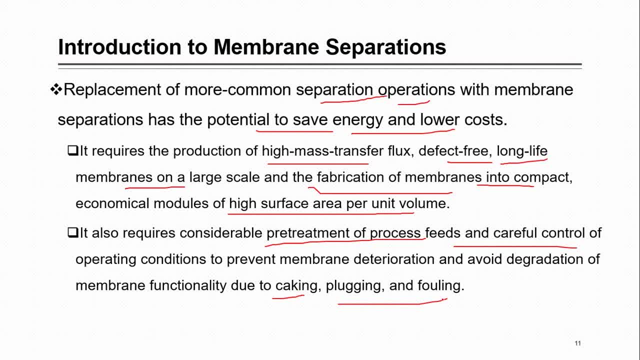 membrane. So membrane should be such that it did not allow these cake formation as well as plugging and fouling, because if this takes place, this will definitely deteriorate and degrade the quality as well. it will create difficulty in the separation, because if some cake is formed on the surface of membrane, maybe you will need now more pressure to pass. 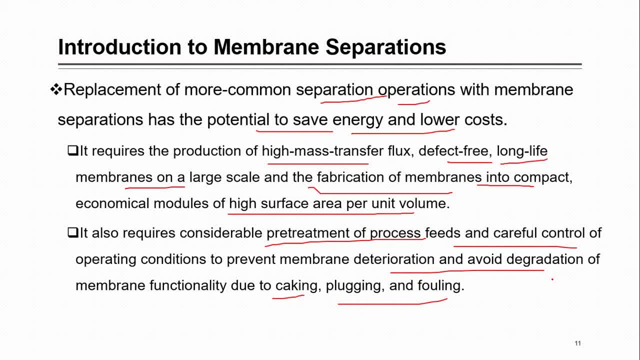 your liquid through this, So that will add on operational cost. So in order to avoid those problem, membranes are being designed in such a way that these problem can be minimized. I mean, you cannot eliminate them, But you can also eliminate them by using a. 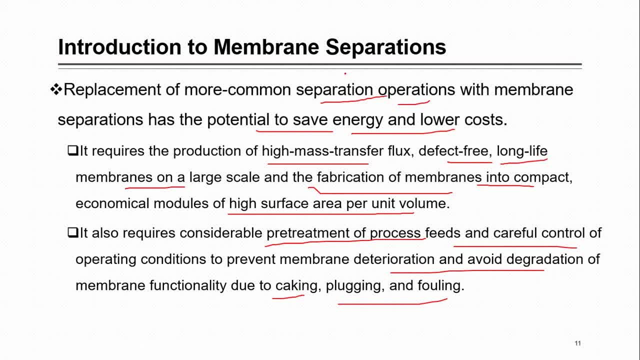 membrane and you can reduce them. So these are some requirements which can help us to replace all other separation processes with these membrane. If we can design some membrane which allow good selectivity, good flex as well, they are in, long lasting, they can be. 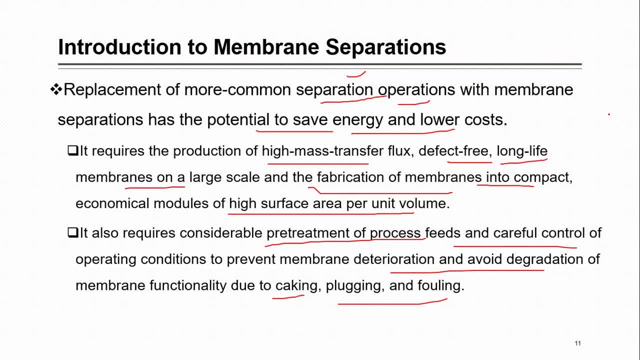 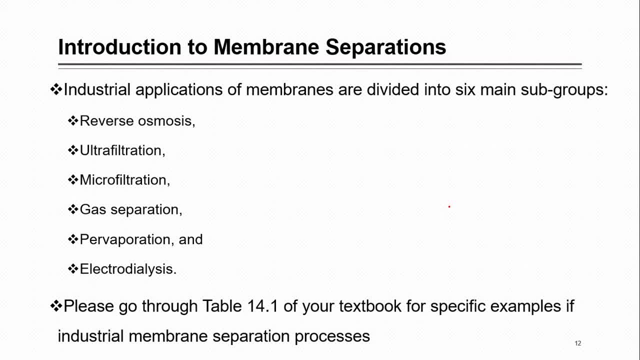 compact and they did not allow the formation of these plugs or cakes on its surface. So, overall, when we look at the industrial application of membrane, So they can be divided actually into the 6 subgroups and those subgroup include: like there is reverse osmosis, then ultra filtration, micro filtration, 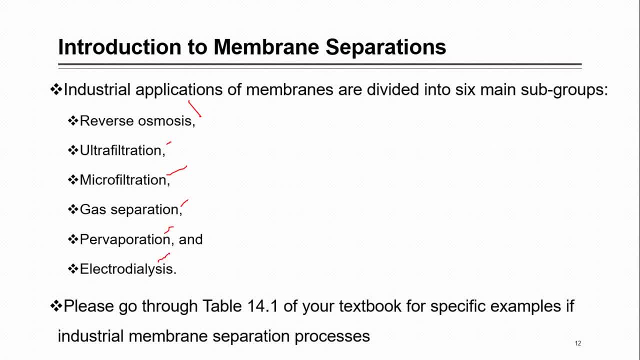 then there is gas separation, pervaporation, and then electrodialysis, And actually all these are used for some specific application. So kindly go through the table 14.1 of your text book and there you will see specific industrial example for all of these membranes. 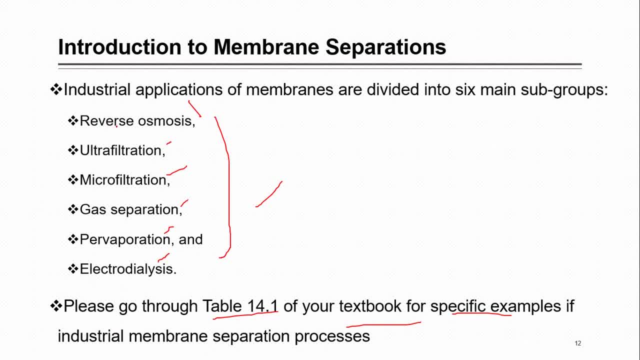 I mean categories. you will see that they are being used from for some specific application. all of those. He has provided us various example that this is used for this purpose, this purpose and so on. So overall, like, for example, if we say gas separation, So that is used for. 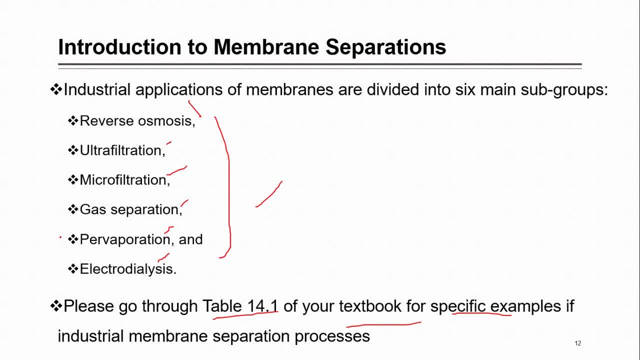 like natural gas separation as well. where are? there are various other examples of its industrial application. So reverse osmosis that is used for usually water. I mean cleaning in the form of, like, maybe, water growth, So ground waters even cleaning as well, like sea water. So many other you will look at. 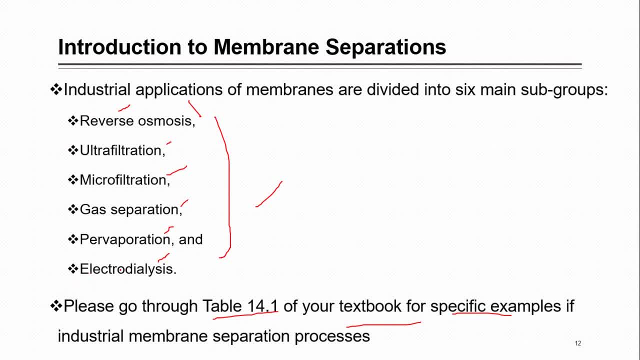 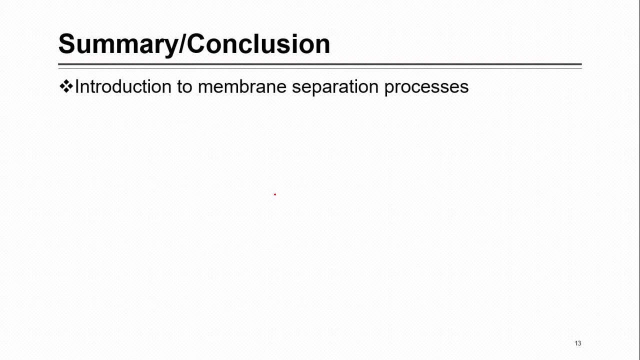 I mean for all of these techniques. So kindly go through that table and just remember few of those, for example. at least you should remember one of one or two for each of these techniques. So that is it up to here. actually, today I have introduced you only with the ground water.